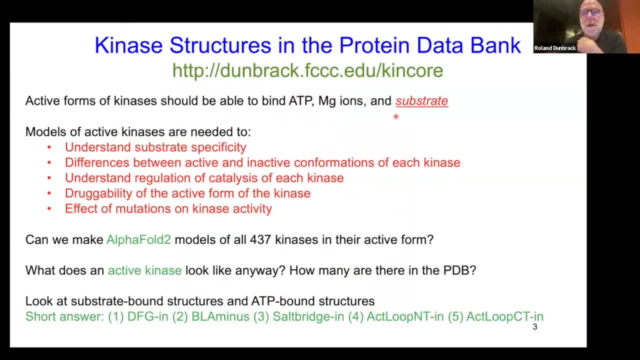 active forms of kinases. They should be able to bind ATP, magnesium ions and substrate, And we want active models and as well as inactive models. but for the active models, we want to understand substrate specificity, And so you need to know what the active structure looks like, what the 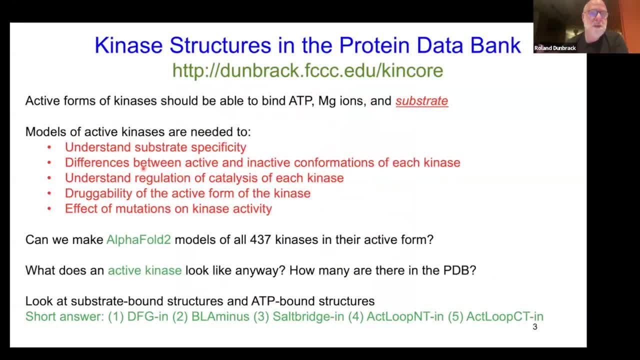 substrate binding form looks like. We want to know the differences between active and inactive conformations of each kinase. We want to be able to understand the regulation of kinases. what makes the kinase active? phosphorylation or binding other partners? the drug ability of the active. 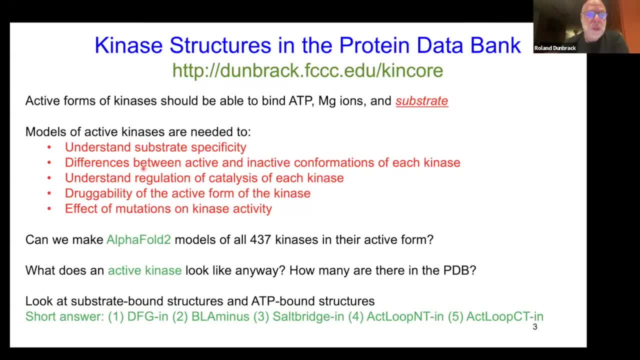 form of the kinase and the effect of mutations on kinase activity. So a mutation might make the inactive state less stable, it might make the active state more stable, And so we need to know both the active and the inactive form. And so we want to know: can we make alpha-fold make? 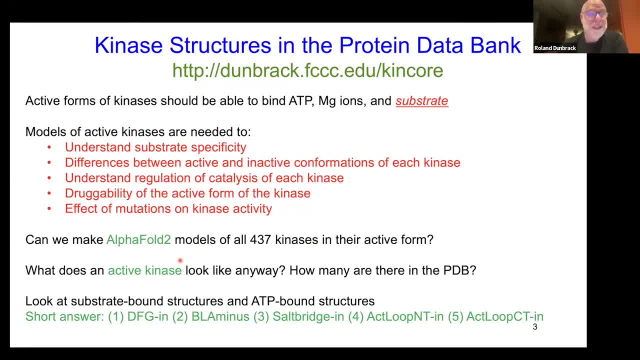 models of all of these kinases in their active form. What does an active kinase look like, anyway, and how many of them are there in the PDB? And the way we did that is to look at substrate bound structures and ATP bound structures in the PDB to get a good idea of what active structures look like. 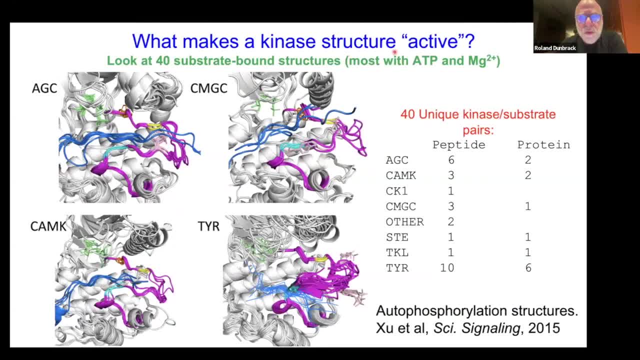 And so, oops, I'm going to close this little link. hold on, there we go. what makes a kinase structure active? And what we did is we looked at 40 unique substrate bound structures in the PDB, that is, different kinases and or different substrates, And here are pictures of those. 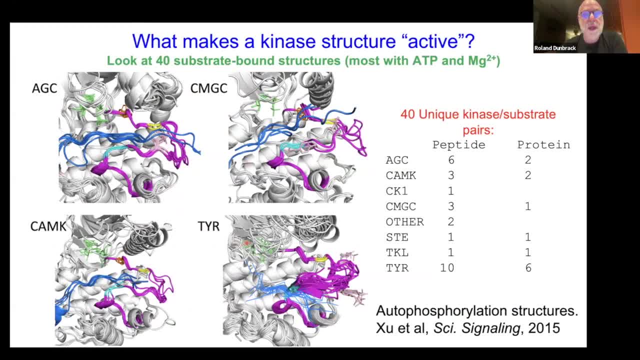 from the AGC kinase family, the CMGC kinase family, the CMK and tyrosine kinases, And they all have some kind of common features. One is that the activation loop here is in magenta. It always starts here at the DOG motif. 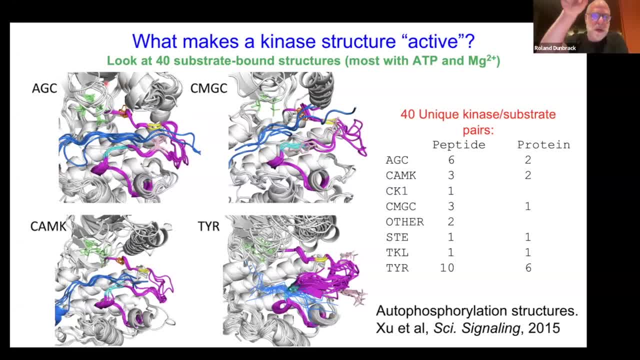 and extends to the right. We always look at kinases with the N-terminal domain at the top and the C-terminal domain at the bottom, So it always goes all the way over to the right and then comes back below, And the substrate here is in dark blue and is in the middle of. 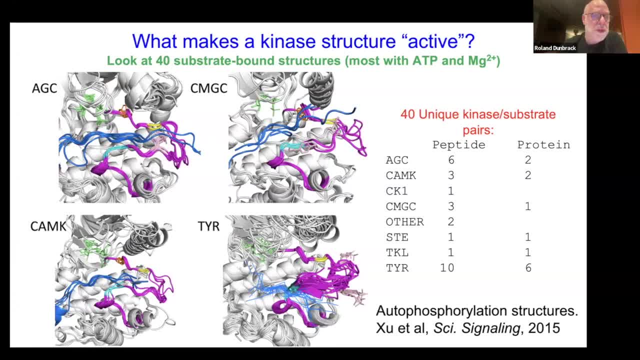 the activation loop, the top part of it and the bottom part of it. The FG motif is up here, that's in orange, And I've marked a couple of other residues that I'll talk about later. These are phosphorylated residues, here in pink And there's one shape. 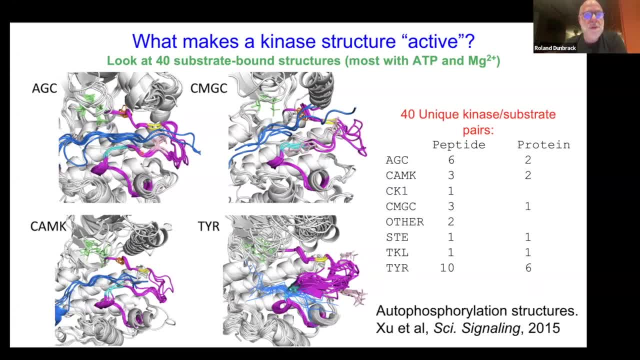 that's very interesting is this sort of upside down bottom boat that you see in AGC kinases. you see in all serine 3-anine kinases. It's a little different in tyrosine kinases But it's the same. you know, that is the same as this shape here and this shape here, if you can follow. 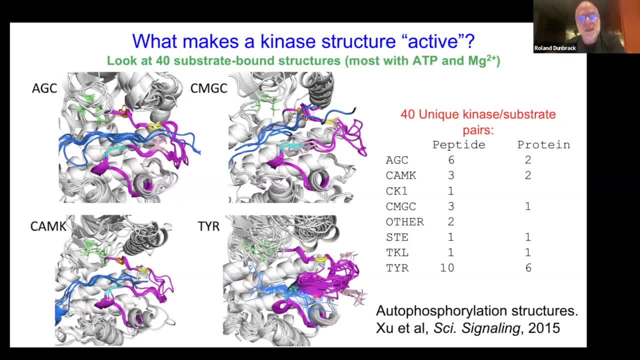 my mouse. It's different in tyrosine kinases, where the position of the substrate is actually different. The substrate binds to the C-terminal part of the activation loop, whereas in the serine 3-anine kinases- most kinases- it's kind of in the middle of the activation loop. Here are just some. 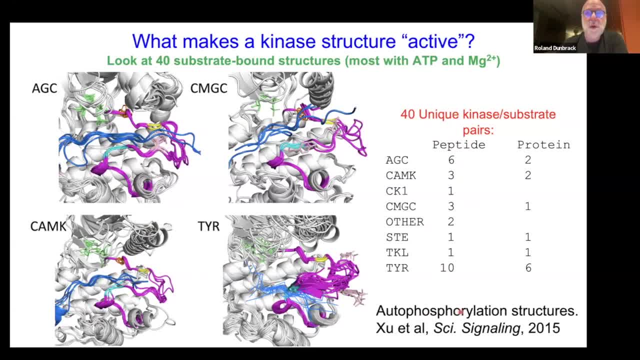 statistics. These 40 structures include some autophosphorylation structures. Those are structures in the PDB where an autophosphorylation site of one kinase, like a serine, 3-anine or tyrosine, is sitting in the active site of another kinase, in the same crystal, in the same kinase. 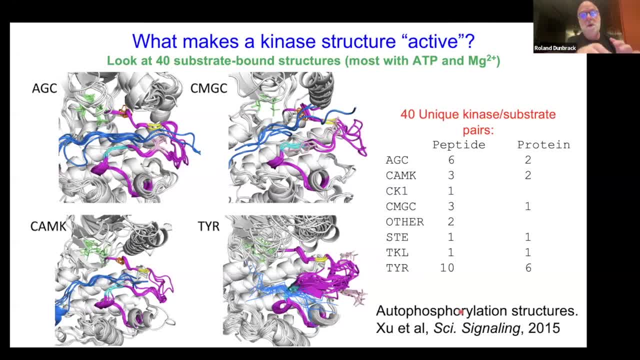 type And that site is an autophosphorylation site. So you can see that there's a lot of autophosphorylation site, a known autophosphorylation site, And we did a study of those eight years ago. 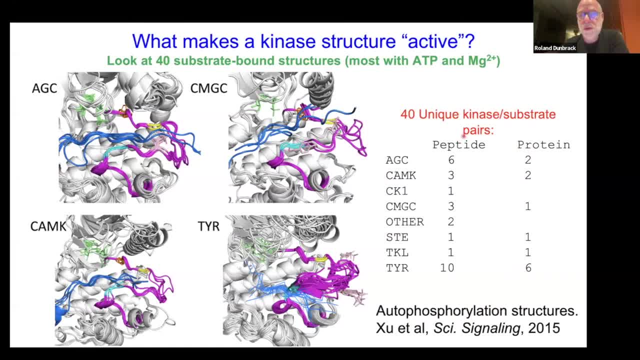 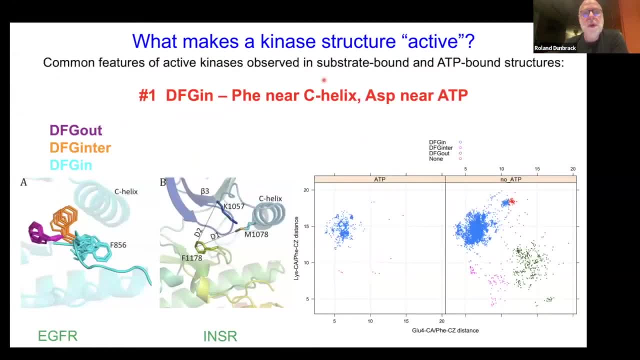 published in Science Signaling. So that includes some of these 40 structures, includes that set. If we look at these 40 structures and we also look at ATP-bound structures, the first thing we notice is the position of the phenylalanine and the aspartic acid of the. 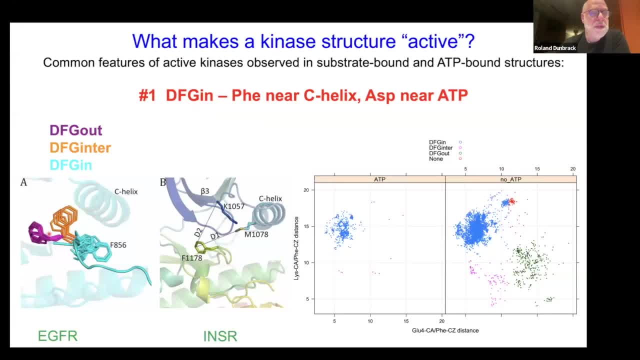 DFG motif. And so if we look here on the lower left, this is the phenylalanine of the DFG motif And we can see that they're basically three clusters of positions. Some of them are underneath the C-helix, Some of them are out of that pocket altogether and way over. 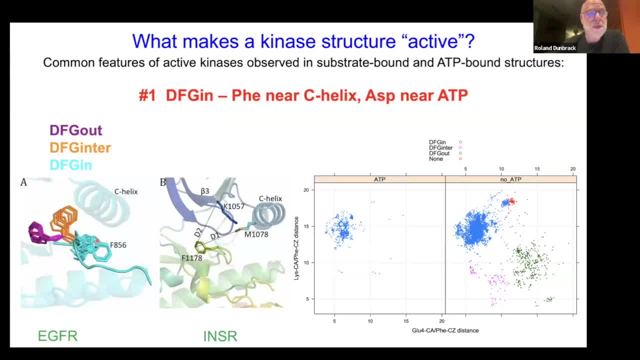 here in magenta, And then some of them are in between, And so these cyan ones are DFG. in The aspartic acid would actually be right where these purple phenylalanines are and would be in the active site, And the phenylalanines are in this pocket underneath the C-helix. The magenta ones are called DFG-out. 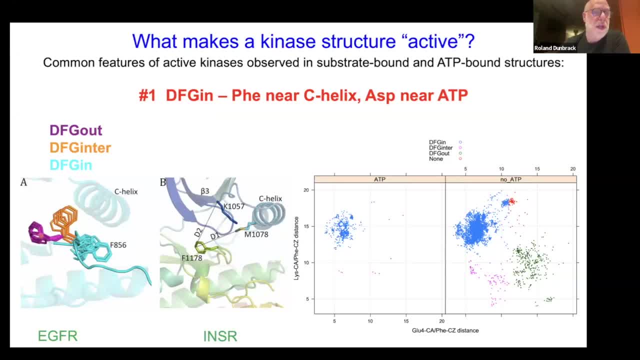 That is, the aspartic acid has been flipped out of this position and the phenylalanine has replaced it. And a few years ago we did clustering of all of the conformations of kinases in the PDB and we used a couple of distances to define what was DFG-out, what was DFG-intermediate. 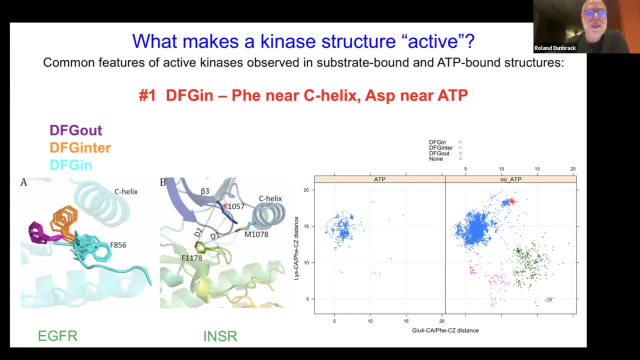 we call this intermediate set and DFG-in, And those two distances are to the lysine glutamic acid salt bridge in the N-terminal domain. So one of the distances is to the lysine C-alpha. The other distance is to a residue, that's four positions after the glutamic acid of this salt bridge. 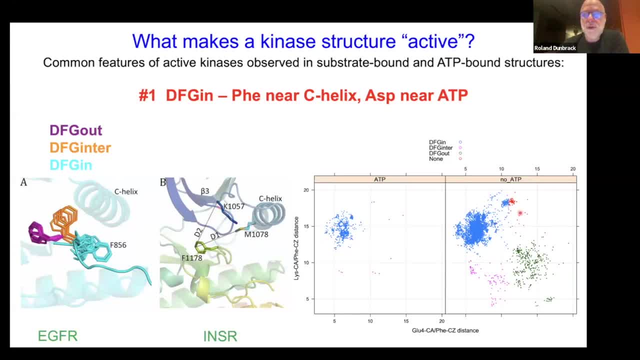 so we call it Glu plus four And if we look at all the structures in the PDB that do not have ATP, you see a really broad distribution. These blue ones are the DFG-in structures. They're the ones that the phenylalanine is very close to, this methionine here, this Glu plus four residue. 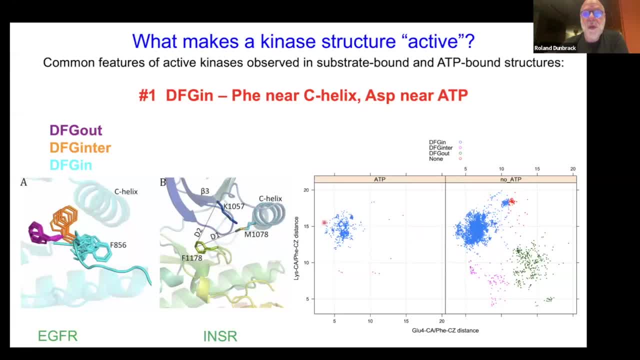 and far away from the lysine. And if we look at only the ATP structures, they are almost all DFG-in, So they're the two. And if we look at only the ATP structures, they are almost all DFG-in, So they're the two. 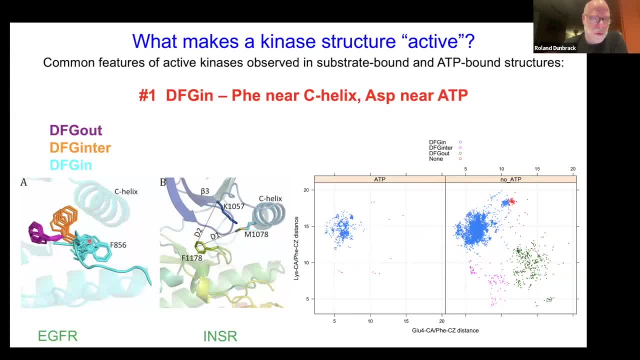 So they're the two, But we do not have the rest of the tests yet And you may want to compare those And you may want to consider these dfg in. so they're that, they're this, you know, kind of position where the phenylalanine is here. 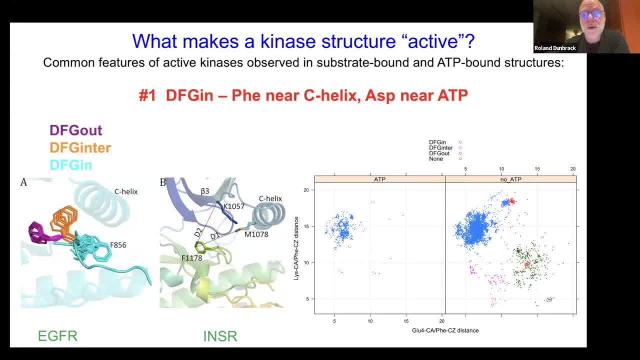 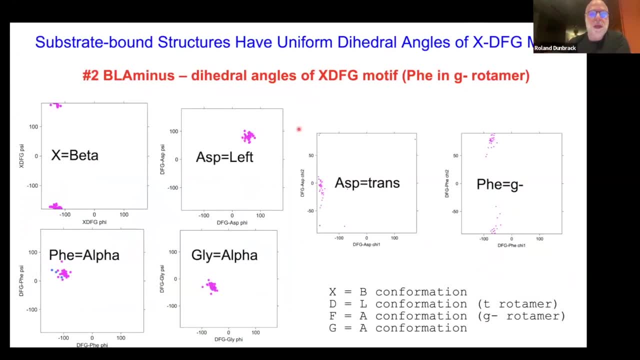 um, these green ones are dfg out. that includes type 2 inhibitor bound structures. um are the green ones over here? um, if we look at the dihedral angles, that position, that phenylalanine, as well as the, the x, the d and the residue before the phenylalanine, uh before the dfg motif. 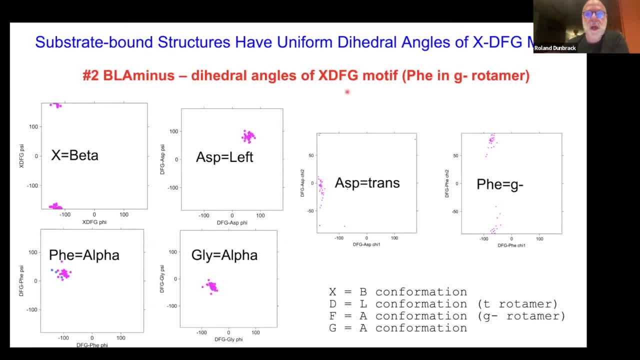 the d, the f and the g um- these are what the dihedral look like- of the 40 structures that um, uh have substrate bound, these 40 unique structures, um, and they follow the same pattern all of them. so the, the residue before the dfg, if we call it x, um, is in the beta position of. 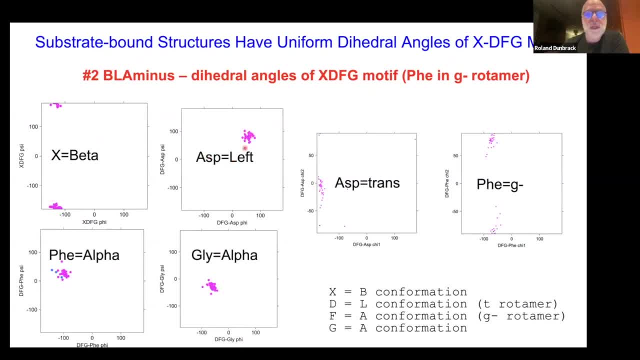 the ramachandra map. um. the aspartic acid itself is in the left-handed part of the left-handed helix part of the um ramachandra map. proteins don't actually have left-handed helices, but um but it would be in this left-handed side. um. the phenylalanine is in the alpha region. 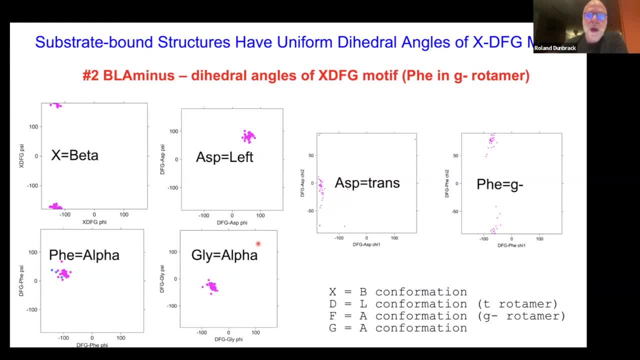 and so is the glycine, but actually slightly different positions. and then if we look at the dihedral angles of the side chains, the aspartic acid is um, has a trans chi one dihedral and a zero degree chi two dihedral, and the phenylalanine has a g. 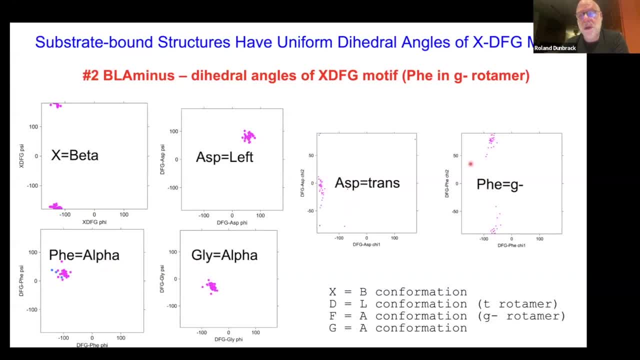 minus uh chi one dihedral and about 90 degrees uh for chi two, as it usually does, and so we call this conformation b, l, a minus, and that's after the x residue is in the beta, the asp is in the left and the phenylalanine is in the a region and the dihedral angle, the chi one rotamer. 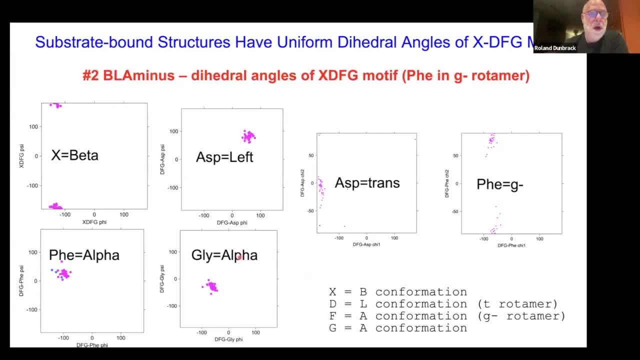 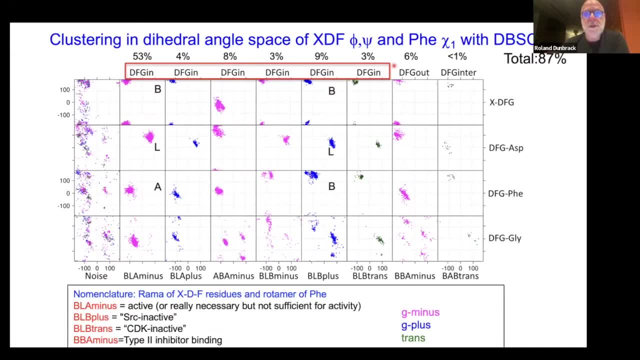 phenylalanine is minus, so that's b l a minus um. i'll show you in a second why we didn't cluster on the, on the, on the glycine. so if we take all the structures in the pdb and we cluster based on just those that set of dihedral angles, um, so excluding the glycine, um, we get this following set of: 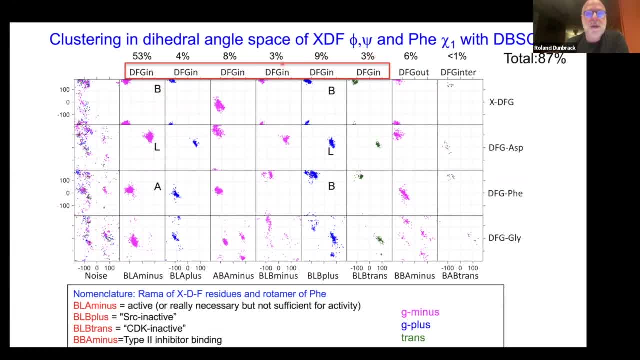 clusters. we get eight clusters um. six of them are dfg in, and so we're going to name them again after the regions of the ramachandra map. so this is b, this is l, this is a, and the color represents the minus dihedral of the phenylalanine um. if we look at some um inactive states, one very common. 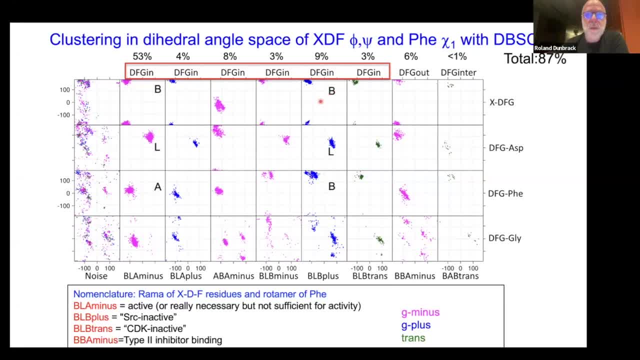 one is sometimes called stark and active um. it's this one where my my mouse is hovering um, and it is b l, b and it's a plus dihedral, and in that plus dihedral the phenylalanine kind of points upwards, pushes the c helix out. it's an inactive conformation of the kinase um, and you can. 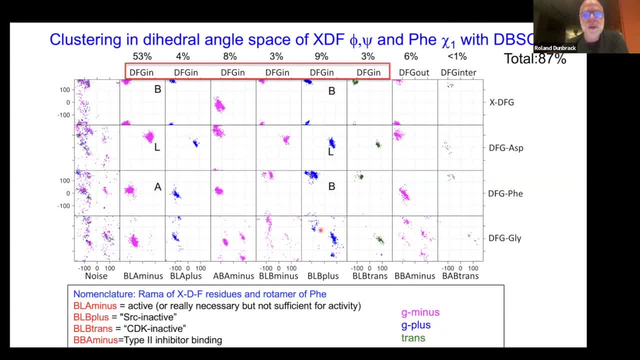 see that the glycine actually in. you know, for some of these clusters there are several different glycine confirmations and so we excluded the glycine, because if you include it you end up with about 30 different clusters instead of eight, and it's really sort of too many. 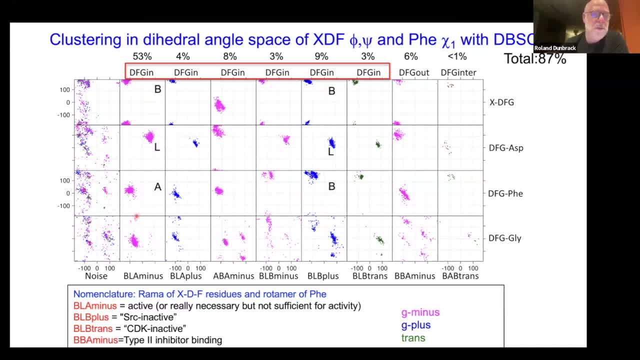 um. but these are the active structures, these are the ones that have atp bound, they have substrate bound, or the b, l, a and the minus um. dfg out ones are b, b, a and minus is a common confirmation for type 2 inhibitor bound structure. so this is stuff we published a few years ago in pnas. 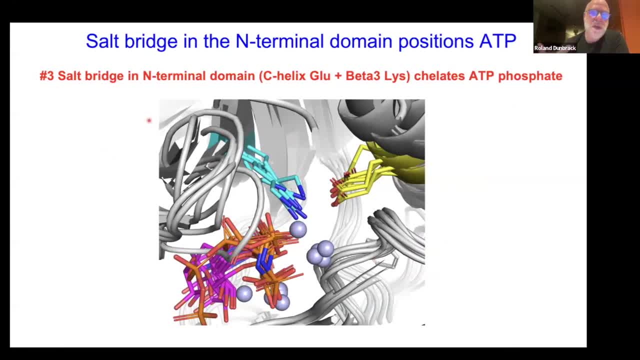 um, the next, the third, so we have dfgn, we have bla minus. the third criterion for active structures is a well-known feature of of active structures is a salt bridge in the n-terminal domain that i mentioned earlier, and so it's a lysine in the beta-3 strand, it's a glutamic acid in the c helix and they make a salt. 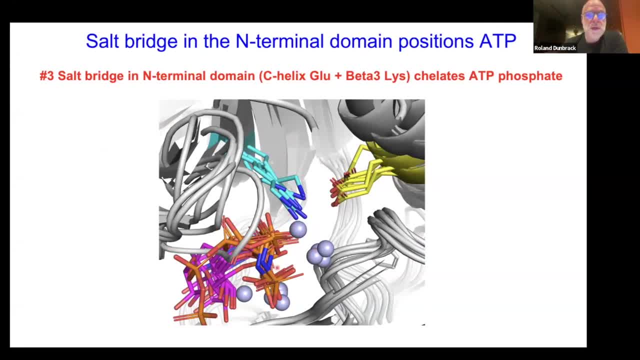 bridge that helps to chelate uh, magnesium ions, as well as the, as well as the atp, and so this is from some of the substrate bound structures, this um, and if we look across all these structures, there's a, you know, there's a very good hydrogen bond distance between 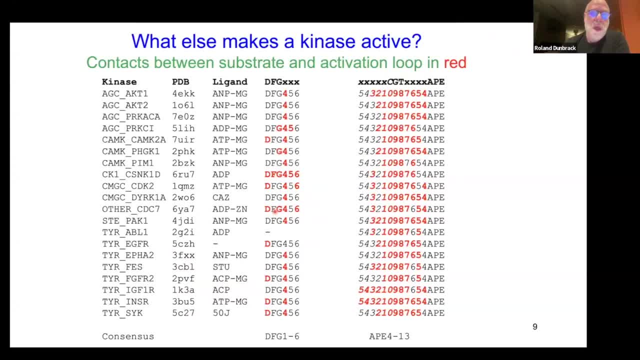 these, these two residues. so that's our third criteria. but the the sort of two new crime- and those are those three are pretty- are well known at this point. um, the next two are ones that we we came to by looking at all these substrate bound structures. so if we look at all the substrate, 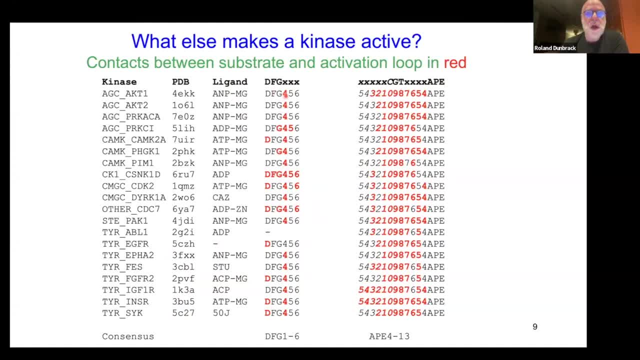 bound structures. we can look to see what are the contacts of the substrate um with the activation loop um, and so this is not all 40 of them, but this is a selection of them um most of them have atp magnesium. if we look at dfg xxx um, the residues in red are ones with contacts of that residue. 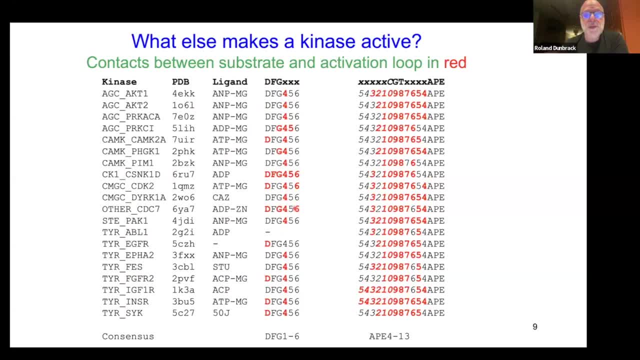 with the substrate. so generally residue four, sometimes residue six, sometimes some of the dfg residues, and if we look at seven, eight, nine- i don't have them printed here, but seven, eight, nine do not have contacts with the substrate, it's really only up through residue six. 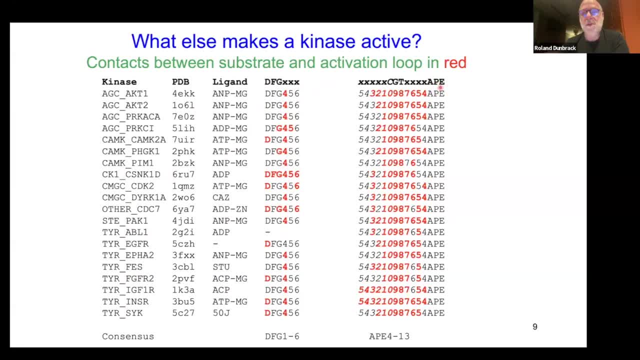 if we look from at the c terminal part, so the c terminal motif is usually ape or spe or ppe. that are the last three residues of the activation loop. the residues that have contacts with the substrate go back to. you know this is residue 10, 11, 12, 13.. um, so they go about as far as residue 13. 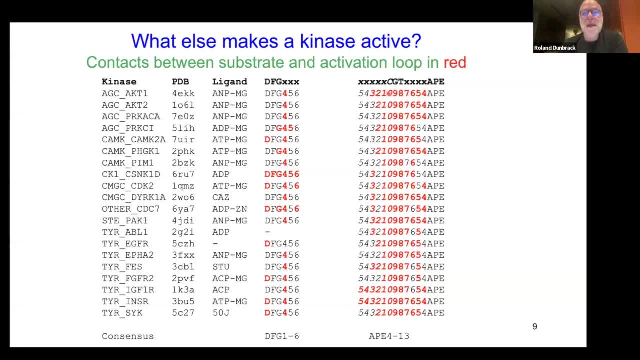 maybe a couple a little bit further um, but definitely in the region of eight, nine, ten. you know, those residues, all, all, almost all substrate bound structures have contacts with sort of eight, nine, ten is uh, ten and eleven, um, and so we wanted to see, well, what are the? 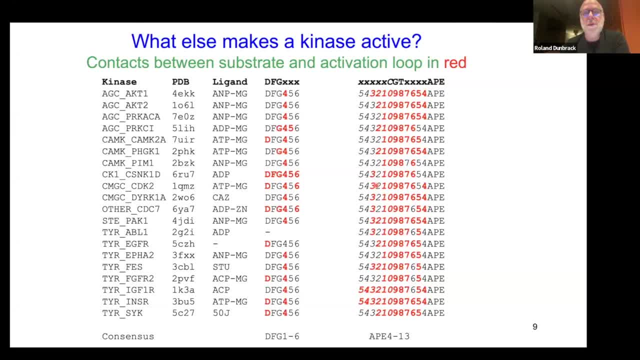 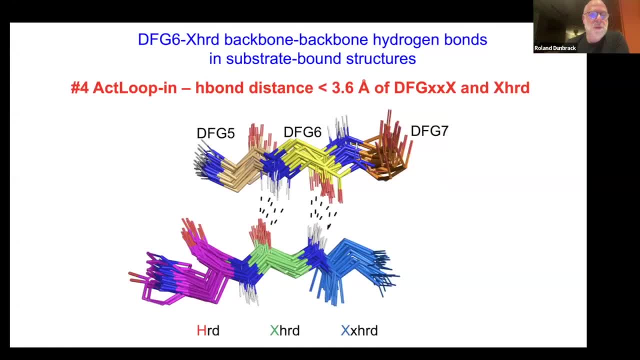 you know positions of those residues that we could you know? what could we use to? what would that tell us about um? you know the structures of active kinases, um, and so the first thing we looked at was um, the n terminal part of it. and if we look at residues, 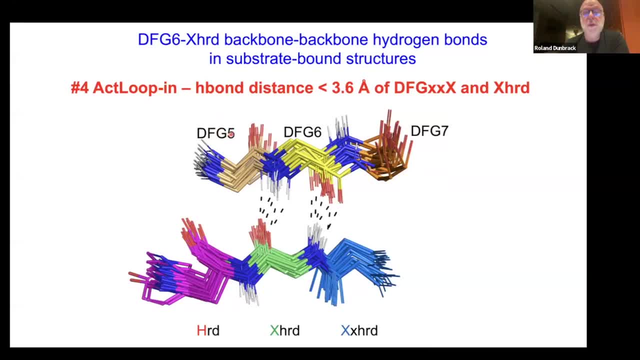 this is dfg xx. so residue five, two, two residues after the dfg, so one, two, three, four, five and then residue six and residue seven. there is a well-known um, hydrogen bond. it's actually a very small beta sheet of a couple of residues um with the xhrd motif. the hrd motif is the act is an. 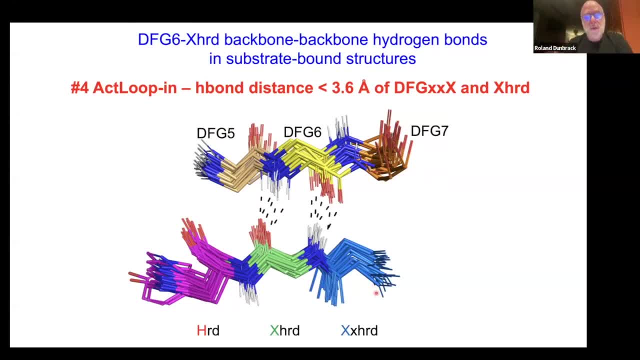 catalytic loop. it's the aspartic acid of the x. the hrd motif makes a hydrogen bond with the substrate, with the substrate oh of the serine, threonine or tyrosine um, and so in all of these um substrate bound structures there are hydrogen bonds between dfg6 and the residue before the hrd. 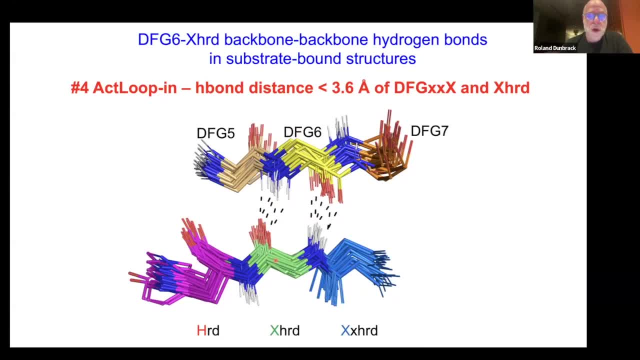 so this is two residues before hid hrd, one residue before hrd in green and then the hrd, and this is the residue in the sequence just before the hrd um, and so that's a very common hydrogen bond. the distances are, all you know, around three axioms, so we set a cut off of 3.6, just to be a little. 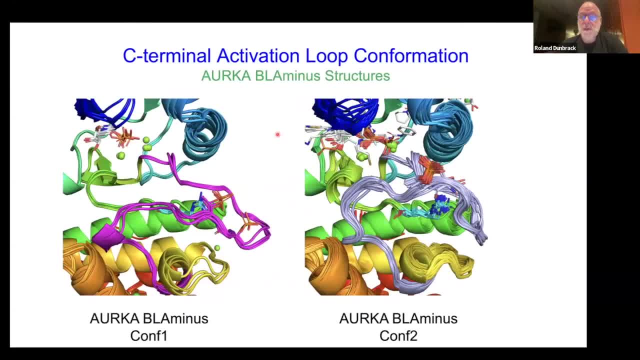 generous, but the other part of the activation loop is. it turned out to be really interesting. if we look at some structures of of, you know, some well-known kinases, um. if we look at aurora, um. if you look at the, the structures that of that are atp bound um of aurora, or and phosphorylated. 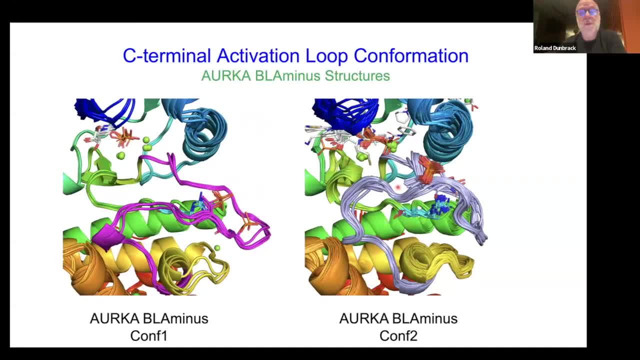 they come in two flavors: confirmation one- we'll call them confirmation one- and confirmation two, um. confirmation one: um has the upside down boat, the. the whole activation loop goes out that way. but confirmation two, um has this kind of double hump um confirmation at the c-terminus and it is. 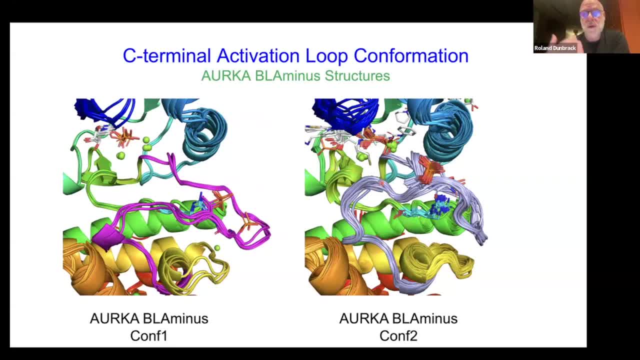 blocking, actually blocking the activate, the active site or the where the substrate would bind um. so these are two very different confirmations, but they are all dfgn, they're all bla- um, they all have the salt bridge and so, and they all have that end terminal hydrogen bond that I just showed you. 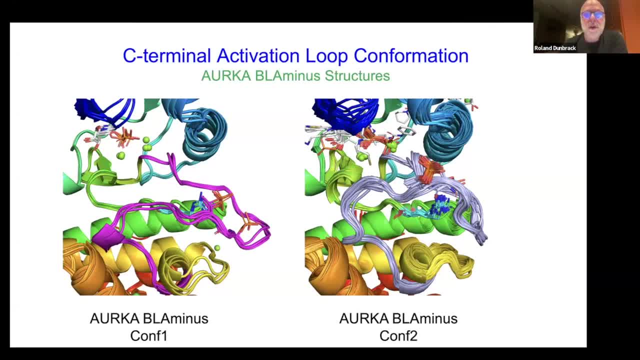 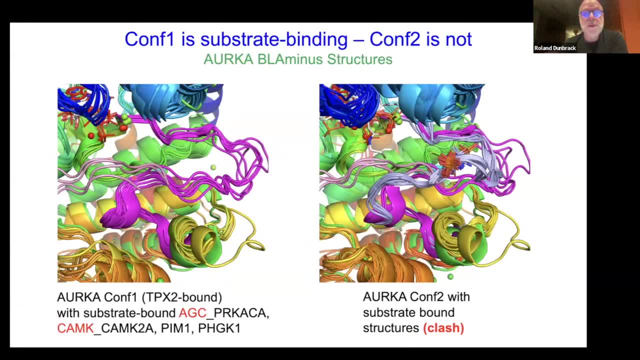 in the previous slide. so we need another criterion to distinguish between these two sets and if we superpose those on structures that have substrates bound, it's clear that. so one of these is the aurora structure, that that is confirmation. one here and several other ones are the are the substrate bound. 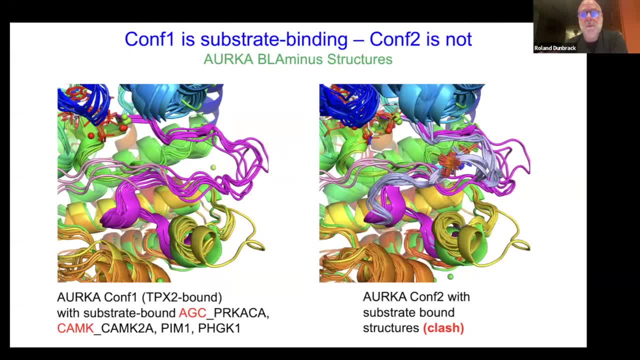 ones, the. it's clear that confirmation one is the substrate binding confirmation, whereas confirmation two, if I put the substrates in, of some structures, there is a big steric conflict between this sort of light, blue or sort of silvery activation loop and the substrates of kinases. 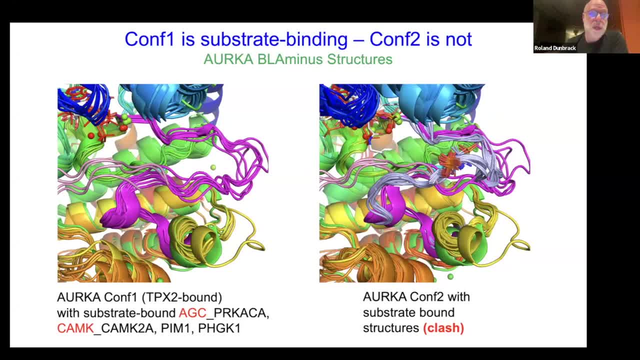 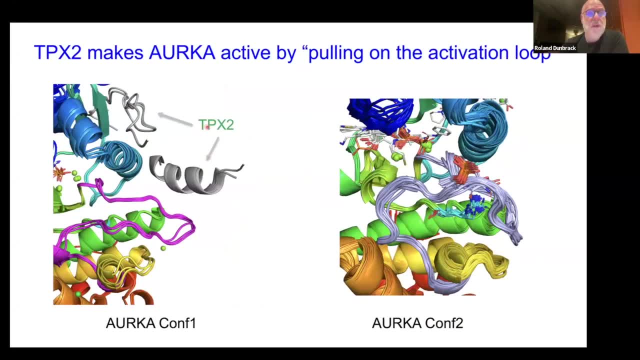 in the same family, and so we need a criterion to distinguish between confirmation one and confirmation two. and oh, by the way, the active structures are bound. have tpx2 bound? basically, tpx2 are bound to the active structures that are bound to the active structures that are bound. 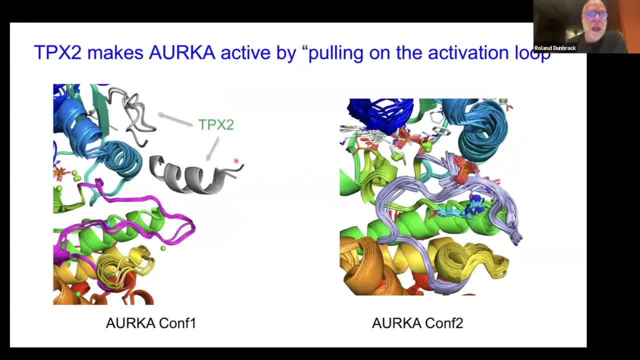 Tpx2 kind of pulls on the activation loop and makes it active. In the absence of Tpx2, it's a little bit like a slinky. The activation loop is kind of bunched up and inactive, And so the criterion that we came to was looking at the ninth residue back from the end of the 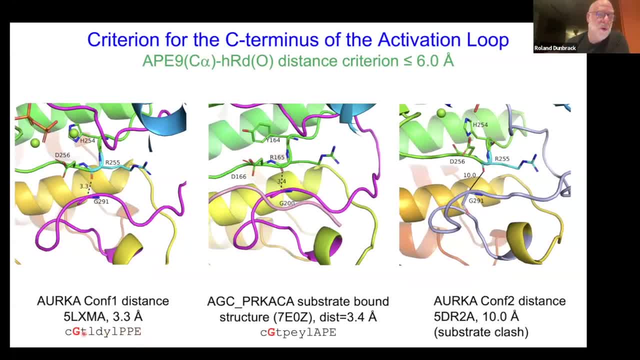 activation loop. So if we count Ape and then count six more residues, there is a very short distance between the C-alpha of that residue and the carbonyl oxygen of the R of the HRD. And so it's sort of it's a kind of a theme that our N-terminal criterion and our C-terminal 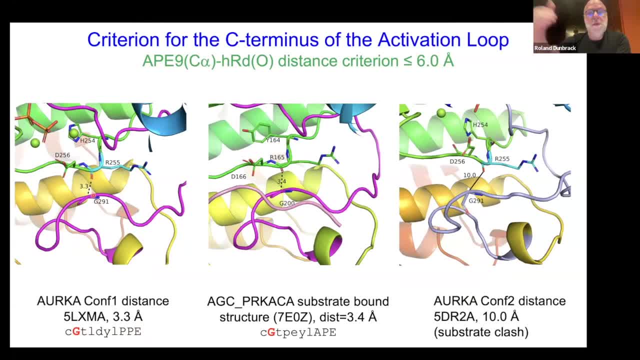 criterion are both interactions of the activation loop with the HRD motif, with residues within the HRD motif, which makes a lot of sense because that's a conserved part of the structure, it's part of the active site and helps to anchor the activation loop in the active form. 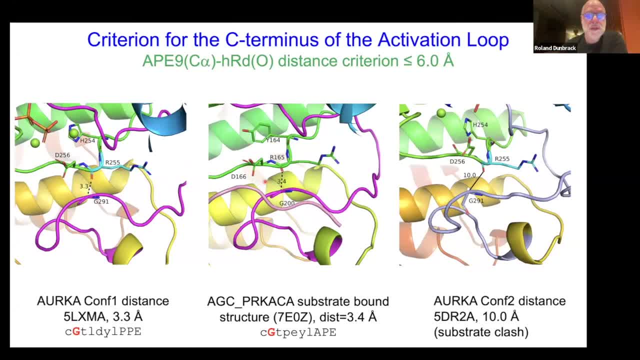 And so that distance is very short in active kinases, in substrate-bound kinases, but it's quite long. Here's our conformation. two of Aurora, and that distance is 10 angstroms, And so we set a cutoff of six angstroms, just based on the statistics. 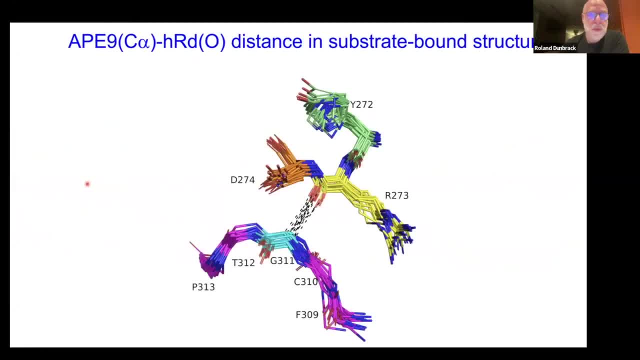 that this distance should be fairly short. And then here it is in a lot of the substrate-bound structures of that C-alpha to carbonyl oxygen distance. And so now we have five criteria. just to summarize: DFGN, BLA-. 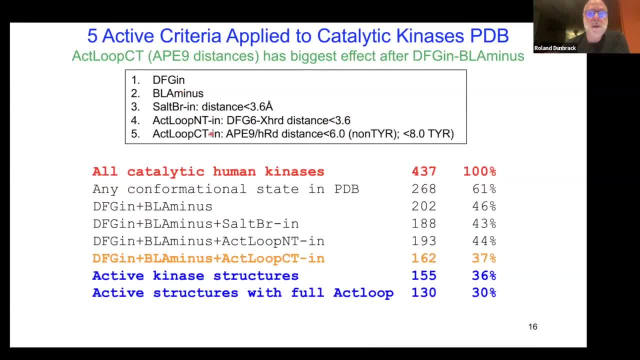 The salt bridge, the activation loop N-terminal and the activation loop C-terminal. Now what happens in the PDB? there are 437 human kinases that are catalytic. 268 of them are in the PDB altogether, 202 are BLA-, 188 are BLA- and have the salt bridge, 193 have the BLA- and 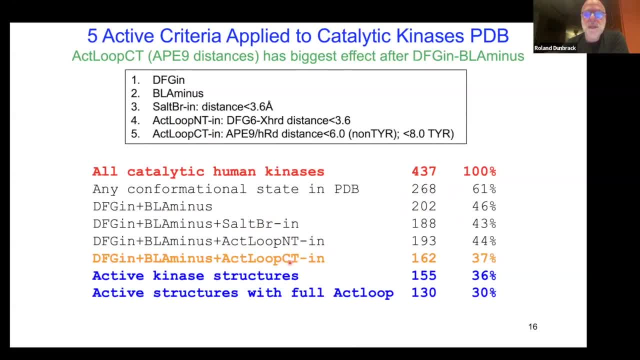 the activation loop N-terminal. I mean there's a big drop when you start to look at the C-terminal. That C-terminal criterion actually eliminates 30 kinases And so if we use all five criteria, 155 of our 437 are active in the PDB, or 36%. 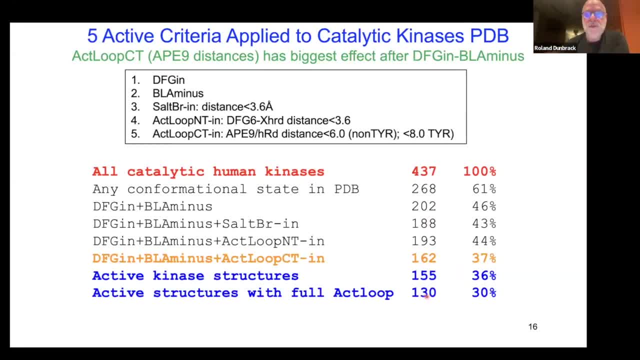 If we look for the entire activation loop, we wanna make sure that it has full coordinates. It's down to 130. So only 30%, And so we'd like to make models of the rest of them, And so we did what a lot of people have been doing. nothing is particularly unique here. 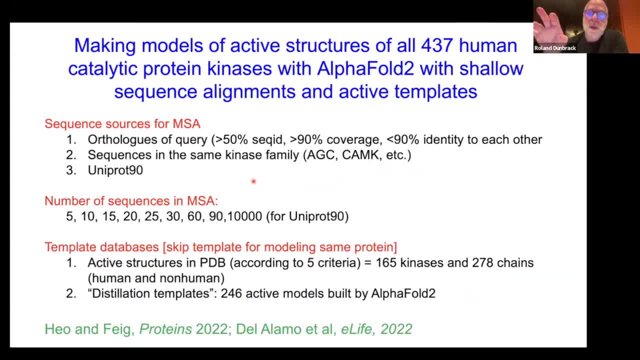 is that we've used multiple sequence alignments for alpha-fold 2. That are shallow- 10,, 20, 30 sequences. And then we've selected templates that are specifically active, That have these criteria that I've just laid out, And so we used orthologs of each query, of each kinase, That is, kinases in uniprope that were: 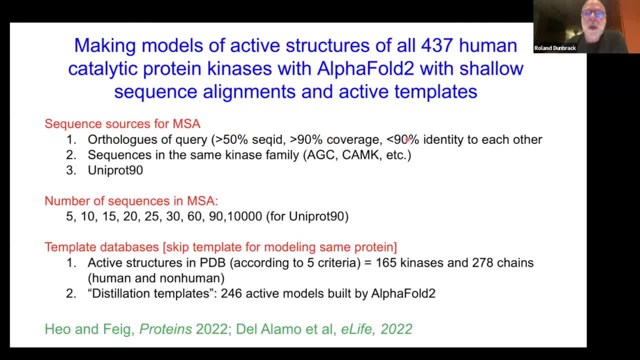 more than 50% sequence identical, that had high coverage and that were less than 90% identical to each other. So we clustered them and picked one from each. We also used all the kinases in the human proteome as another set of sequences in the PDB. 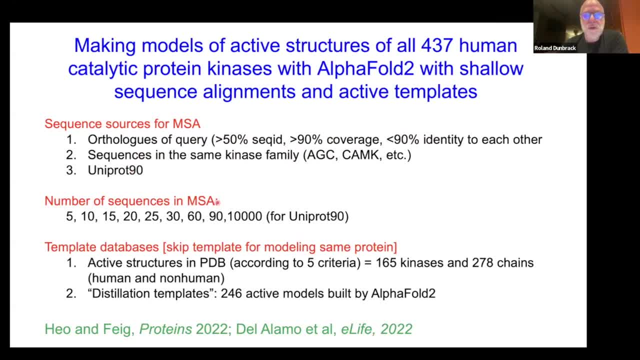 and then we also used Uniprep And we did different numbers of sequences in the multiple sequence alignment, from five all the way up to 90 for the shallow sequence alignments And then for Uniprep we used 10,000.. The template databases we used were we used these active. 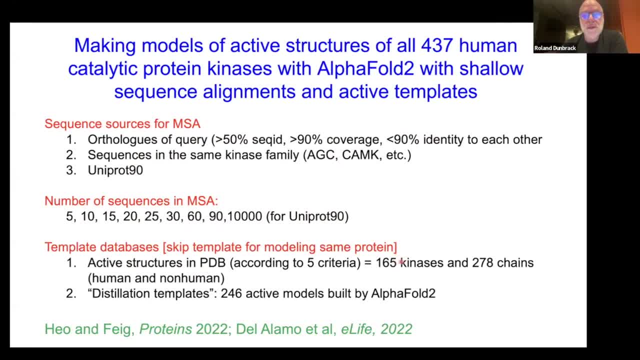 structures in the PDB, including non-human kinases, And so there was a total of 165.. And then we use what we call distillation templates. That is, early on we made models with alpha fold that were active. They passed all our criteria, And then we also use those. 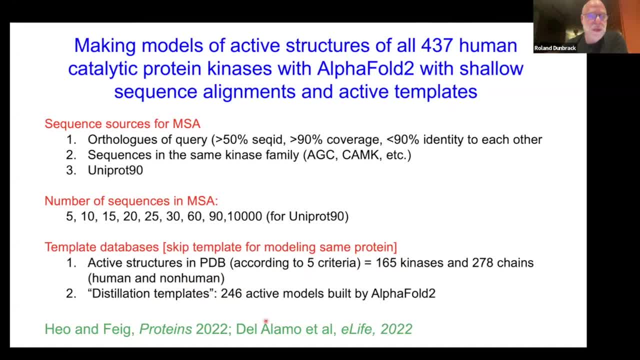 as templates to make additional models. And here are two citations: people that had done similar work on GPCRs or in kinases. you know these shallow sequence alignments on specific templates. This is what happens if. if let's just look at the ortholog set here on the right. 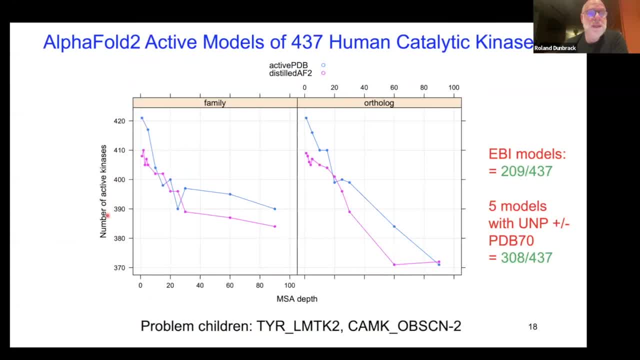 If we the the, the Y-axis is the number of active kinases out of 437.. And as the MSA depth gets lower, from a hundred kinases all the way down to one or two um sequences in the multiple sequence alignment: the number of kinases, the number of kinases for 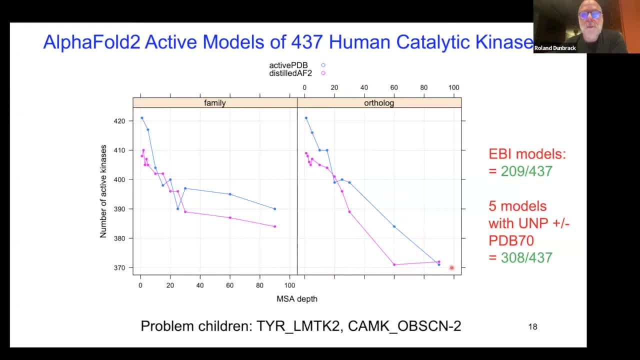 which we get at least one active model rises: Um, and, and these are the two different template sets in the blue and and uh, in magenta. Um, if we look at the EBI website, there's only 209. 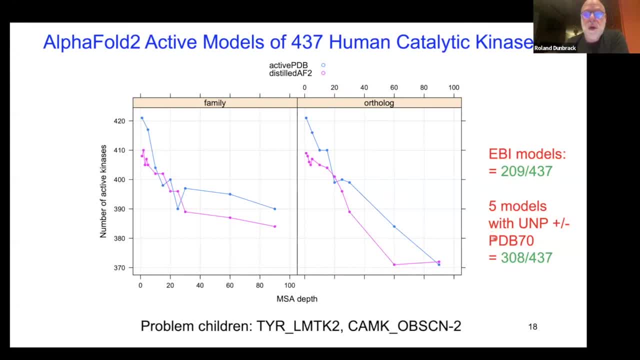 active kinases in that set um EBI's models. Um, if we use five models- you know, alpha fold is five models- with all of Unipro and with PDB 70, um, you only get 308.. So by doing this we managed to get all 437 of them active. What happens is that not any one. 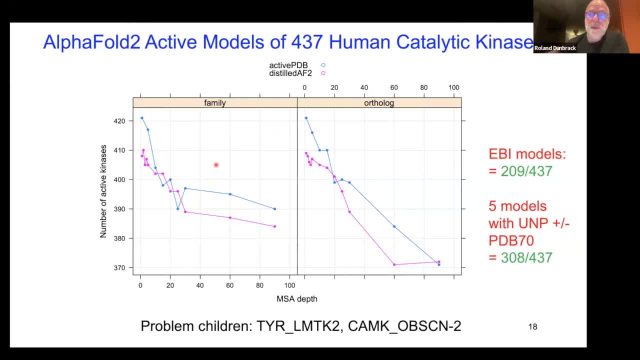 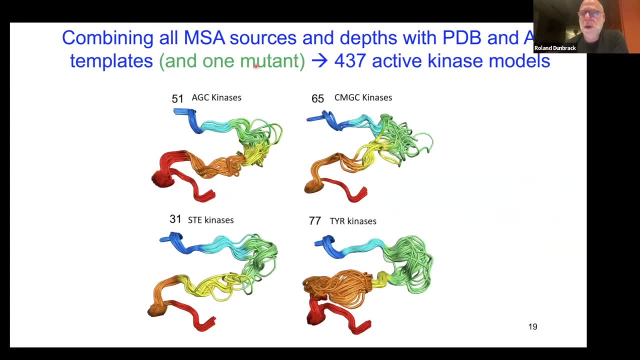 set of uh MSA and templates makes all 437 active. You have to combine the results across all of the different uh MSA depths and template sets, um, in order to get them all to be active. Um, and so we managed to get them all active. We actually had to make a mutation in one of them. 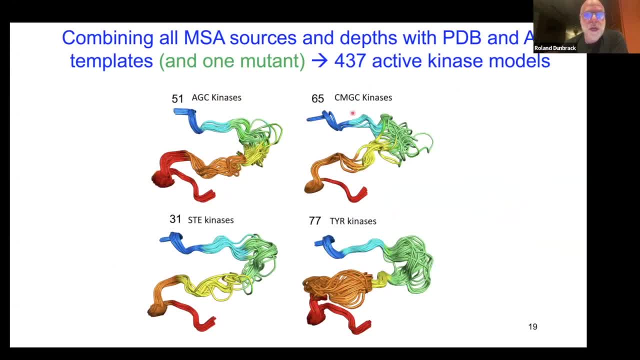 It's possible it's a pseudokinase, We're not sure, Um, but here's, you know, here are sets of these, um, of the structures, Um. so here's 51 AGC kinases. You can see the upside down bottom boat. 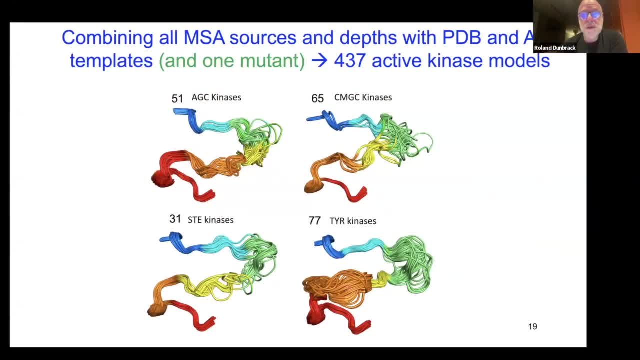 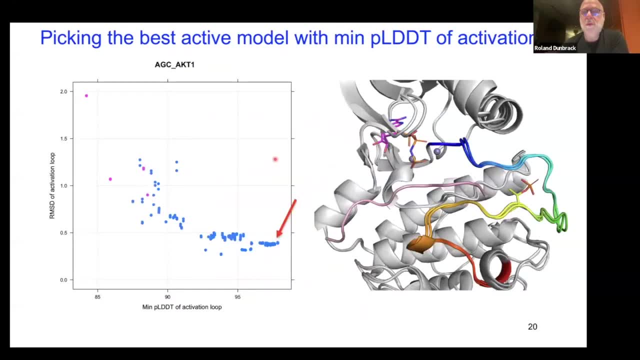 um, same thing for CGMC kinases and then tyrosine kinases. That activation loop is really quite diverse. on the C-terminal lines, Um, we pick the best model, one that we actually put on our website by using the PLDDT. of the activation loop itself, We use the one with the best minimum. 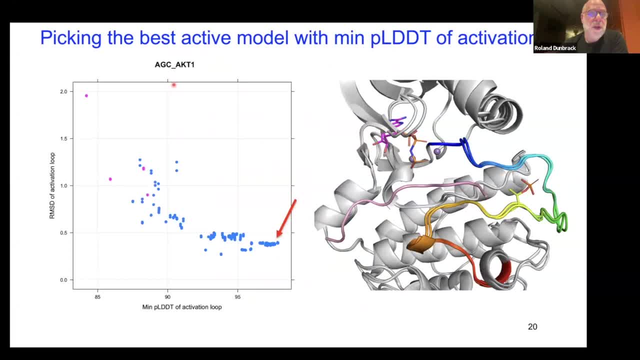 PLDDT- um across the activation loop residues, And so here's a plot of a KT1 with the um activation. These are all different models that we made. Here's the uh- PLDDT of the activation loop. 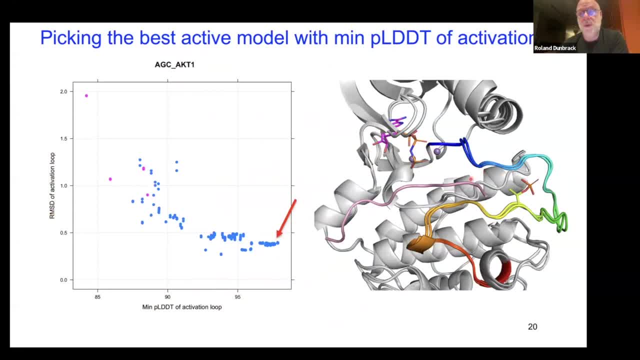 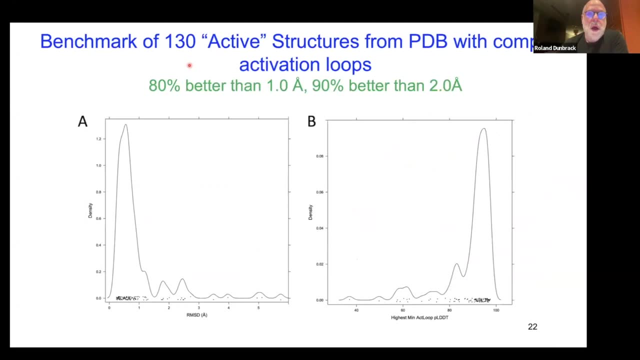 um and the RMSD2, a known structure that has a substrate bound, And so you can tell that. you know, at lower PLDDT you do get some diversity of the activation loop, Um, but the high PLDDT, highest PLDDT structures correlate with the lowest RMSD. That one Um, if we look. 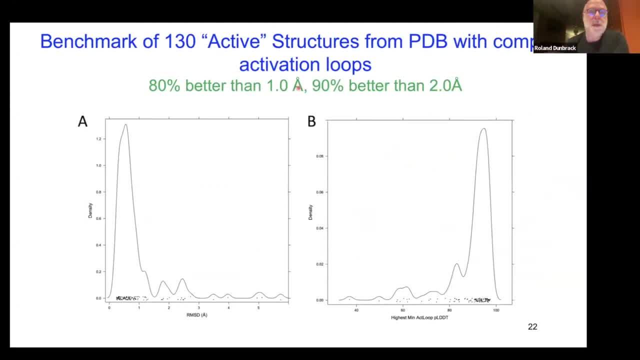 at all 130 of those kinases that have complete activation loops in the PDB in the active form um. this is our RMSD distribution. So 80% of our models of this 130, we have a model that is better than one angstrom RMSD to that. 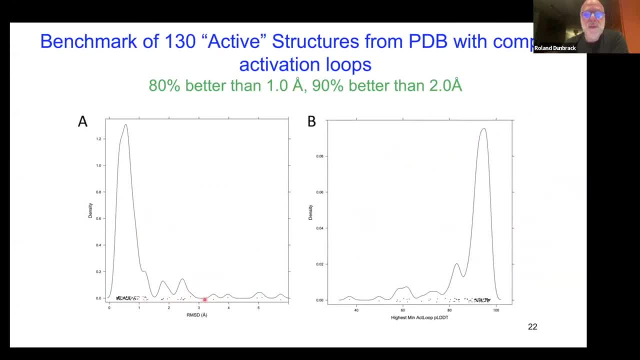 structure. Um, there's a few out here and we looked at a lot of these. Some of them, we think the PDB structure is not fully active, That is, there's some position of parts of the activation, outer parts of the activation loop, that are actually blocking the active site, Um, and so 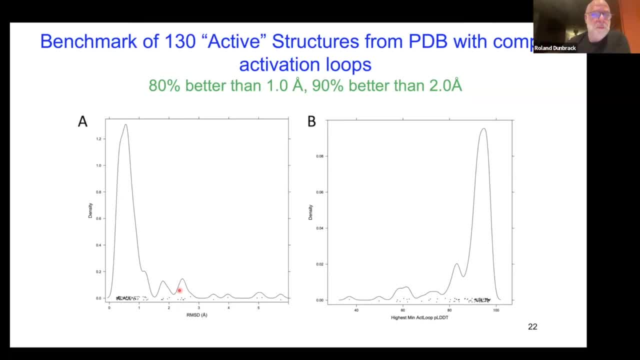 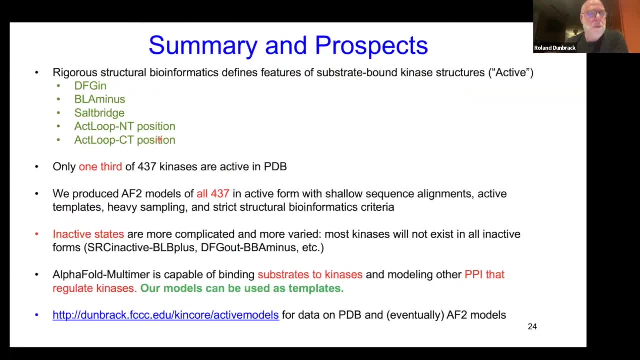 we think our model, most of our models, are pretty good, Um, so let's get that Um. I just want to summarize: Um. these are the criteria that we used for, um uh, active structures in the PD, both, both in the 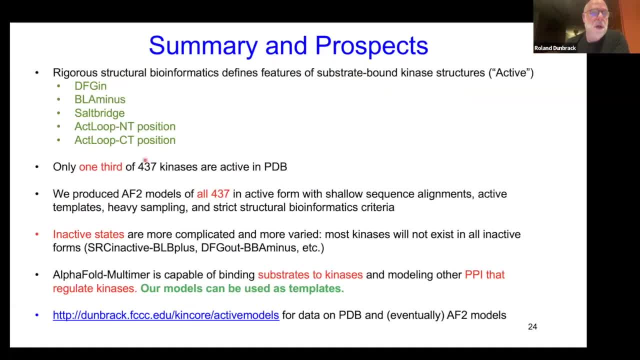 PDB and for, uh, the models that we got out of alpha fold Um, only one third of the hundred of our 437 kinases are active in the PDB, And now we have models that I think are pretty good of all. 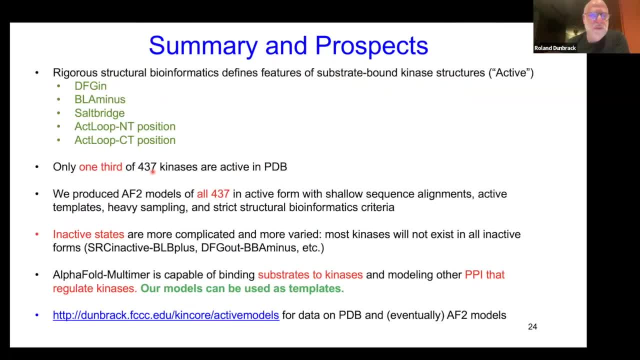 437, um in the active form. Um inactive structures are actually a lot more complicated. Um there are some kinases that have really dominant inactive forms that we would like to get alpha fold to produce those inactive forms. Um other kinases have really broad distributions of inactive 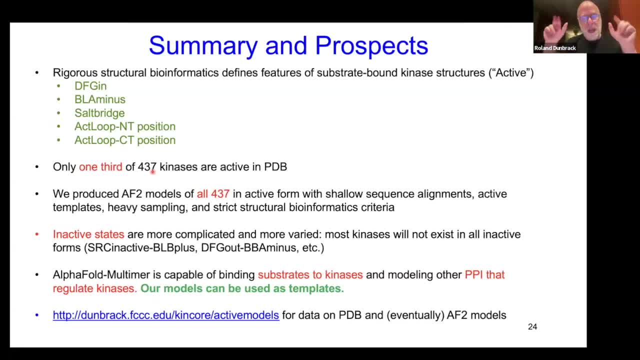 structures and it's not clear what it means to to try to get the inactive form. They may not have as well likely not to have um a single inactive form, but that's actually very complicated. You can make a DFG out structure. You can get alpha fold to make any of the forms of kinases. 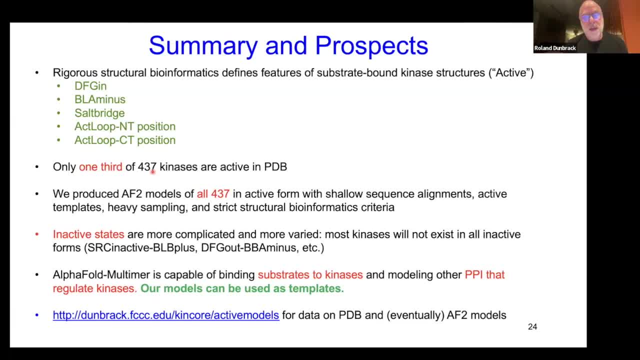 but are those really the dominant ones that you would see inside cells, Or are they ones that are picked out by weird inhibitors or they're just part of the landscape? It's? it's really actually really difficult problem and people have been approaching it, Um, but I think I don't think. 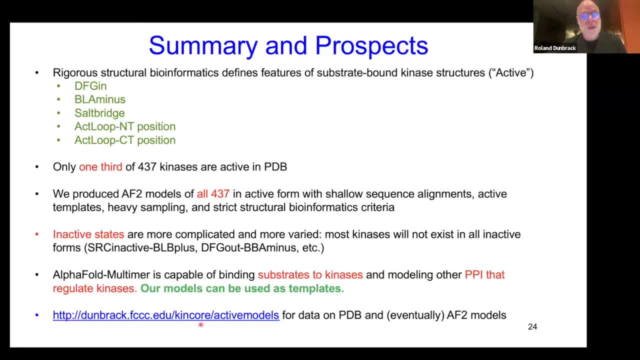 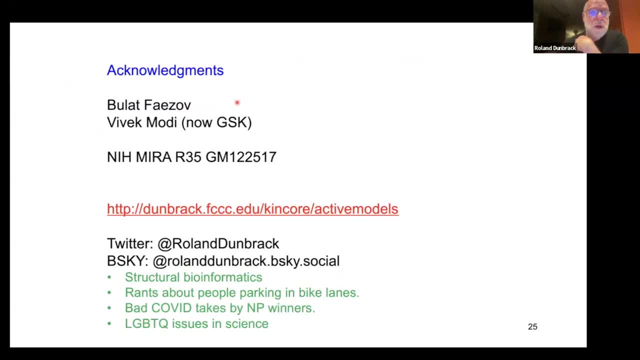 we have an answer to that yet. Um, and then, finally, everything is on our website. um, on on that page. Um, and I want to thank a lot. He's the student that did most all of this work, Um. 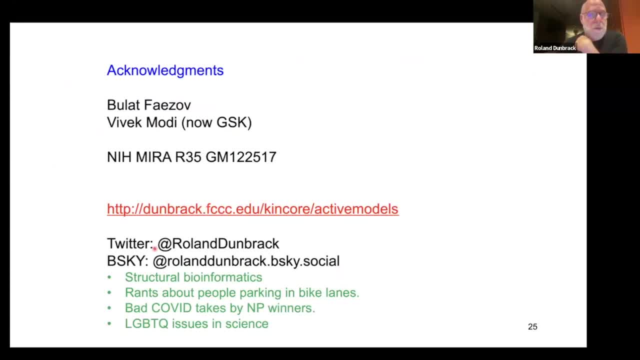 Vivek Modi did all of the early classification of kinases. Um, I'm on Twitter and also now blue sky, which I think is a better place than Twitter. Um, and I talked about structural bioinformatics. I rant about people parking in bike lanes. 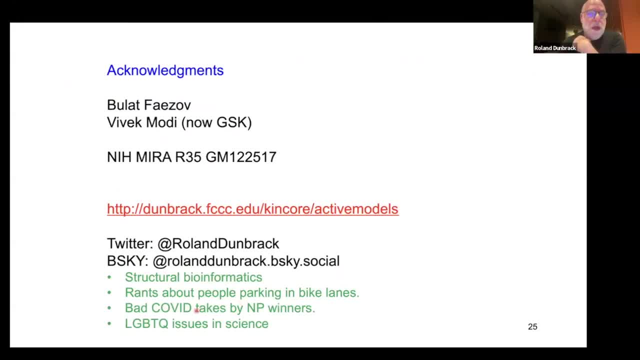 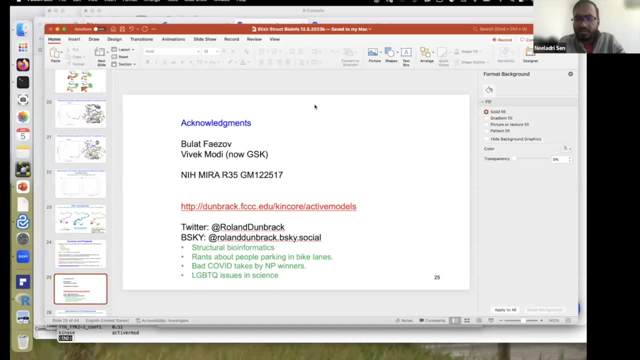 Um, I have an argument with the Nobel prize winner about bad COVID takes, Um, and I talk about LGBTQ issues in science. Um and so with that I will stop and answer any questions. So if you have any questions, just put it in the Q and a. uh, so I guess we have the first one from. 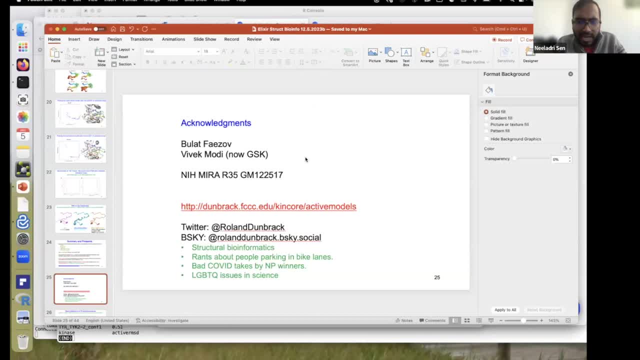 uh. so the first one is: is the key: is activation or deactivation states really shared across, uh, all around the kinases, right, I think? I think the, the, the for active kinases, you would expect it to be shared, or, or you know pretty much all kinases have to have the. 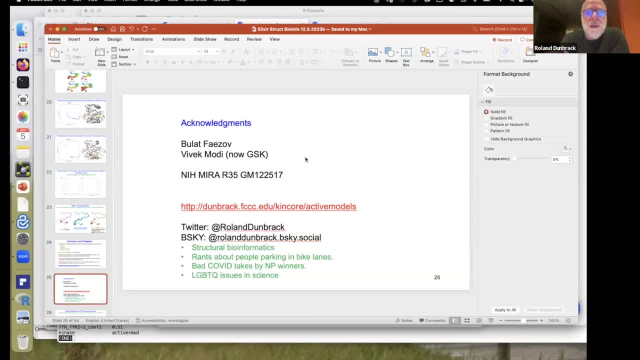 same active form around the active site and you know they have to bind a substrate, So there has to be a groove where the substrate fits. Um, they have to bind ATP, And so we we're pretty confident about the criteria around the active site for the active structures. Inactive structures are: 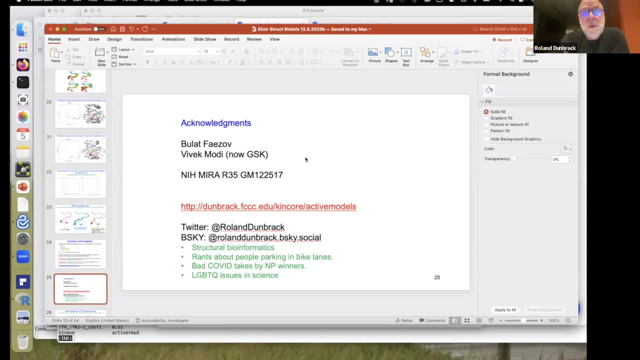 different, It seems. tyrosine kinases for instance. quite a few of them have a kind of folded up activation loop That's DFG out makes a little beta sheet strand and a turn, and then another strand, Um, and then a tyrosine um in that. 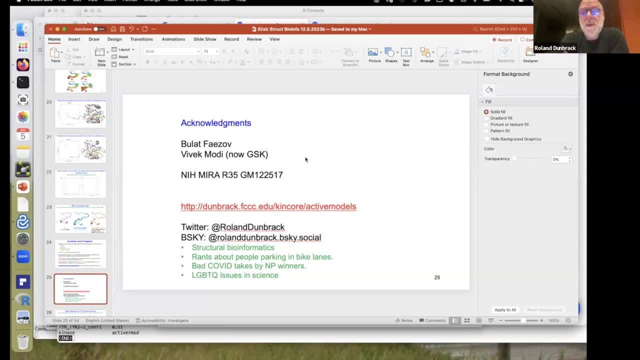 uh beta sheet um makes a hydrogen bond with the HRD motif. So it's sort of auto inhibited like a substrate uh, pseudo substrate Um. but that's not all tyrosine kinases and you can get alpha fold to do that to most tyrosine kinases. but you look at the PDB, look at FGFR structures. 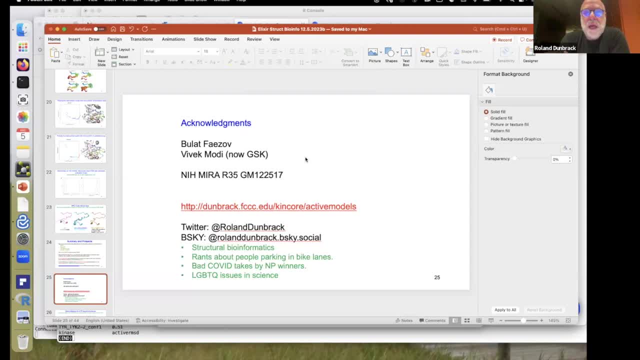 and there are hundreds of them, and none of them have that, That motif, that structure. And yet I can force alpha fold to make that structure. I don't know what that means. I don't know. That means, you know, we're, we're. we're making a fake structure. 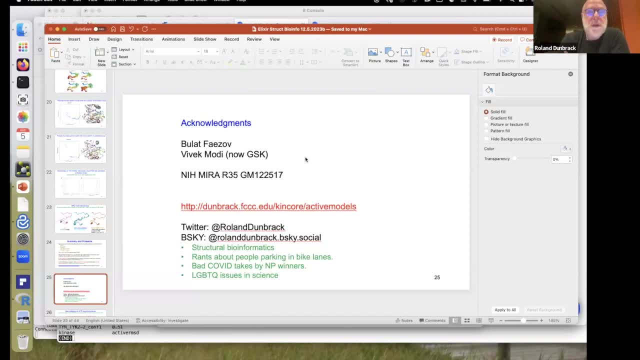 and it's not really what FGFR looks like. or just nobody's done a PDB structure with that FGFR structure. Um agency kinases, for instance, don't really have inactive forms. All of the structures in the almost all the structures in the PDB look active. They are regulated in a different way. 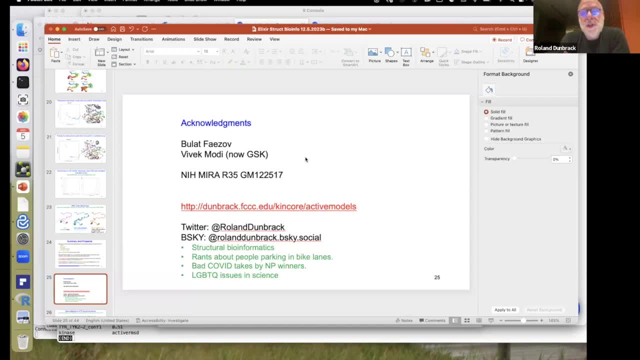 So if you look across the kind of they do not share inactive structures, across the kind of sub families share some inactive forms, but but it's actually really a complicated problem, I don't think we know the answer. A couple more questions, Um, by looking at the kinases. 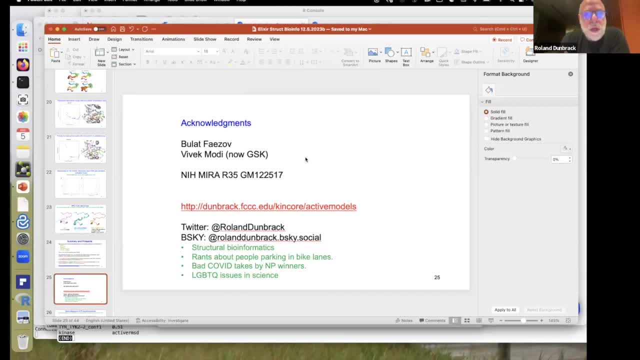 can we predict how other enzymes, that say phosphatases for instance, will behave in similar situations? I think that would be really interesting to look at, to look at different enzymes to see if they have, you know, kind of clustered confirmations of loops in their active. 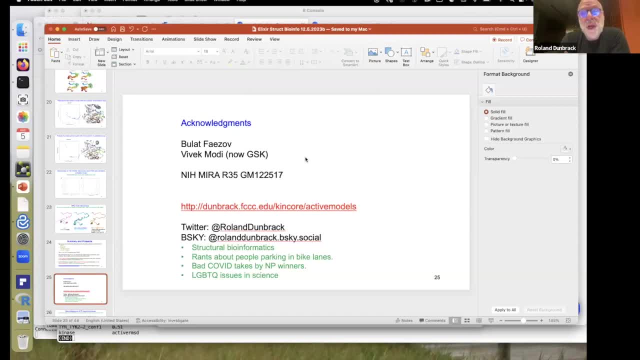 sites. I'm sure people have, you know, one family at a time, Um, but I think I think we could do the same procedure where we get an idea of what they look like in the PDB- what's active, what's inactive- and then apply that to alpha fold as templates. 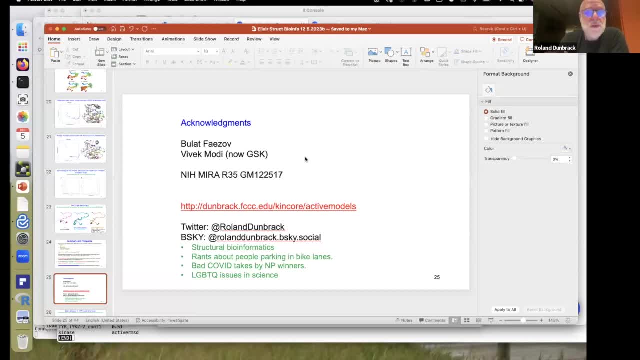 um and apply it to alpha fold as models to try to get, try to get two different states. That would be fun. Uh. next question from Carol is: uh, so when kinase inhibitors developed inactive form should be a better target? I most, I think most, kinase inhibitors are targeted at. 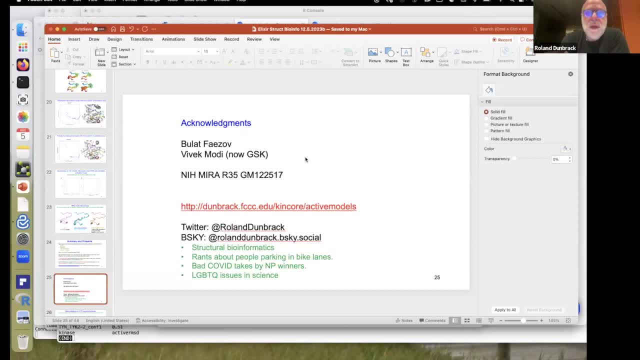 inactive structures, but not all of them. Uh, and you know, if the kinase is in an active state most of the time in cells- some kinases are like that- then you would really only want to target the active form, Like AKT1 is really, you know, just active. or PKA let's use. 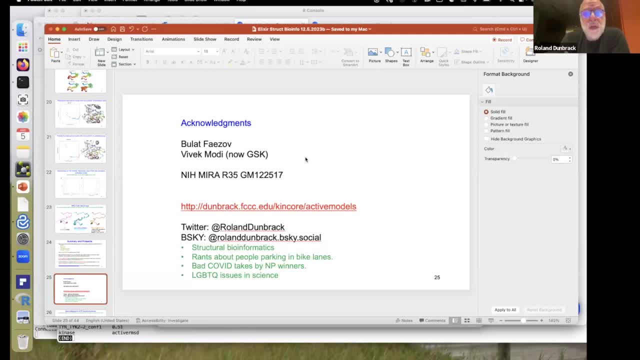 PKA as an example. Um, it's really only active in the in the PDB um and probably only active in cells and is regulated, has regulatory subunits and and uh. PKI is an inhibitor protein for PKA. 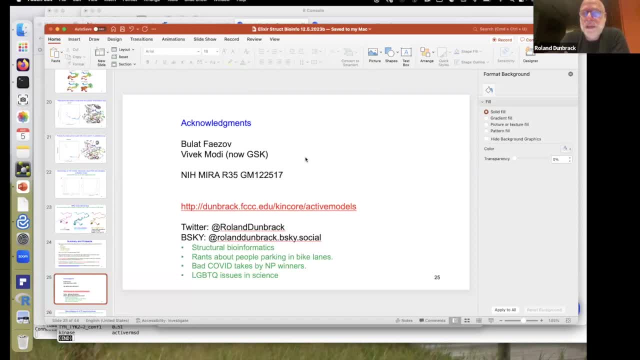 that that Susan Taylor has studied. So not every kinase really has an inactive form and we don't know which ones have stable. you know inactive forms that you would see in cells that you would want to target in the inactive form and which ones don't. So that's an open question. 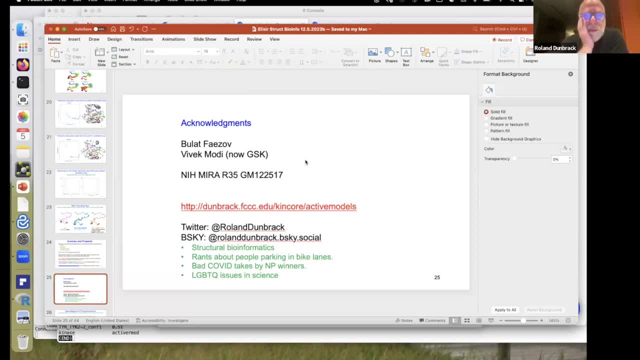 More questions: Um, from Raymond Hackett. some ATPases are only active as dimers, um or large multi domain complex. Is there something similar in kinases? Yes, there is Um. some kinases, uh, are activated by dimerization, like BRAF. Um, and we're actually 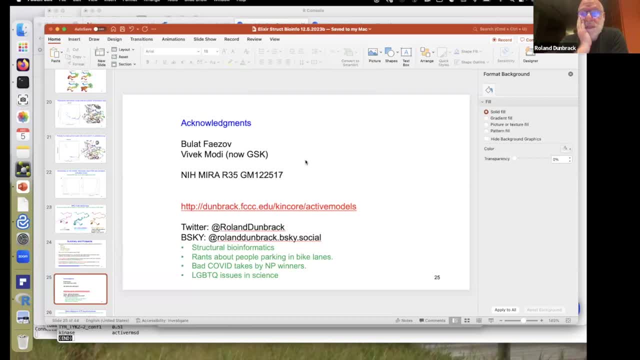 doing a study where we're trying to make homodimers um of all of the kinases and see which, but with AlphaFold, AlphaFold Multimer, and see which ones get good scores, which ones is AlphaFold um strongly wants to make a dimer Um, and there's. 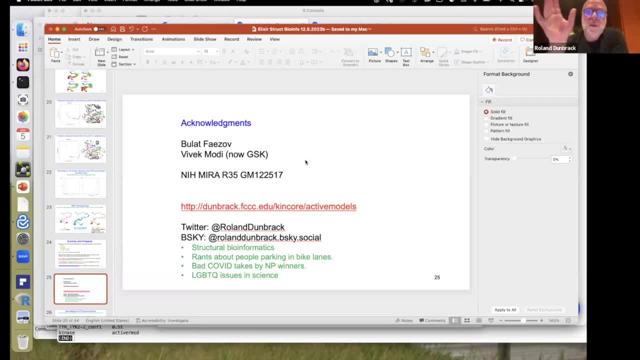 some really interesting cases where it makes dimers for like a small family of kinases And you look in crystals of the, in the PDB of those kinases and the same dimer is present. So we won, for example, Um, and yet none of the we won structures are actually annotated as homodimers. 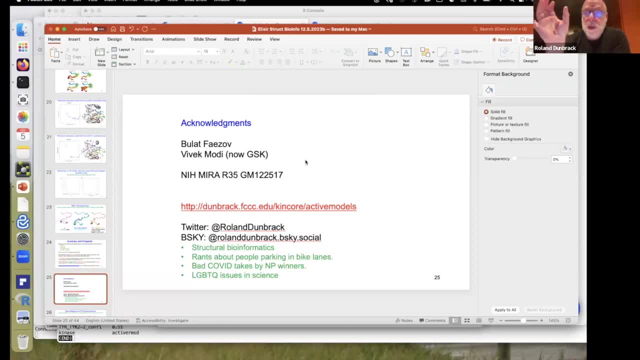 And, as far as I know, Yeah, We talks about, we want homodimer um as a, you know, an active or inactive form of we want, and yet AlphaFold reproduces the crystal dimer and it didn't copy it because it it isn't. 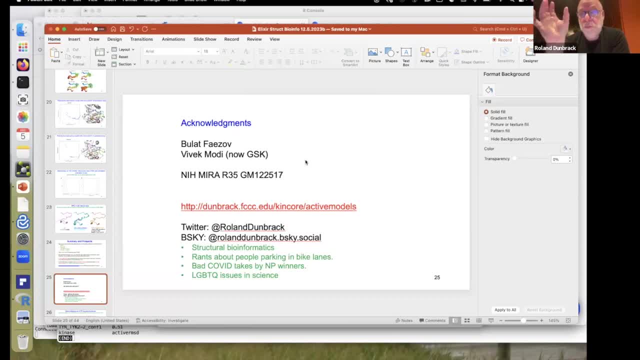 it wasn't trained on that. We won dimer because nobody seems to think it's biological Um, but there is a close family member where there is experimental data that that dimer is biological. It's the same time. So, yes, dimerization is definitely important, um in in the activity. 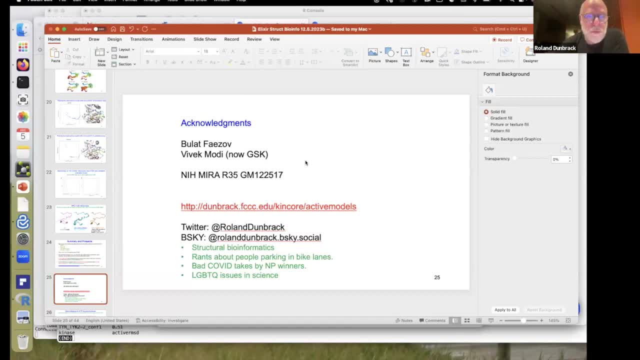 of kinases. Uh, let's see from Vasilis. Would it be possible to use the kinase criteria to uncover other kinase, like enzymes, based on different folds? Uh, there there could be, uh, uh. Janet Thornton, for instance, looks at active sites and looks at kind of convergent evolution of active sites. 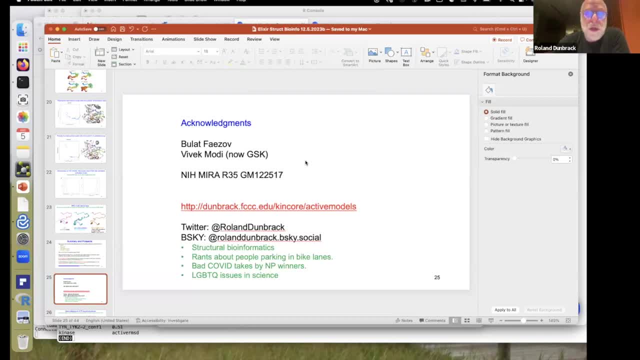 the residues that are necessary for an active site. Um, and so one could use something like that across the AlphaFold database to see: are there? are there proteins that we didn't know were kinases and actually turned out to be kinases? That would be interesting to do. 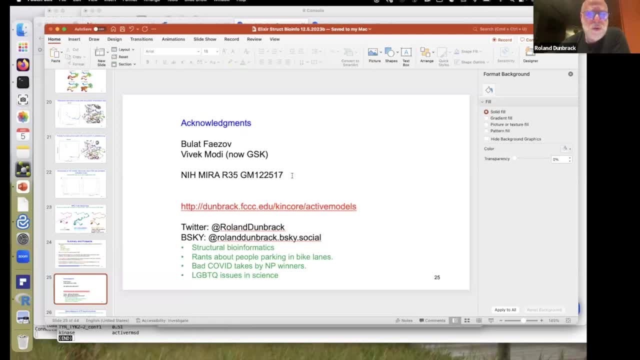 Uh, Mary Navani, what do you think is the role of disordered regions, like a unique domain of SARC? um, interaction with substrate, regulation or activation, Um, all of those things? Um, we have a set of the sequences of kinases from alpha, all the AlphaFold models I looked at. 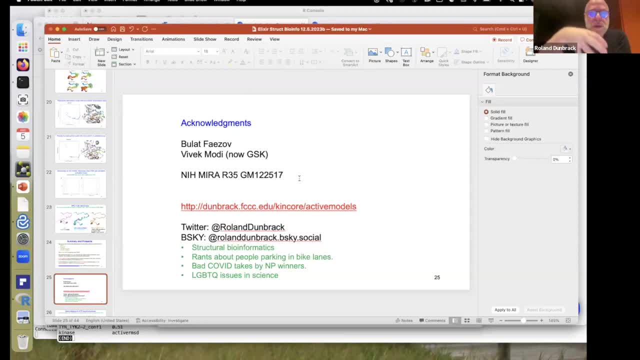 all of them really carefully and found all of the tails. let's see terminal tails, N-terminal tails, adjacent domains that interact with the kinase domain, And so we're using those sequences to make models of all of the kinases that are longer, that are not just 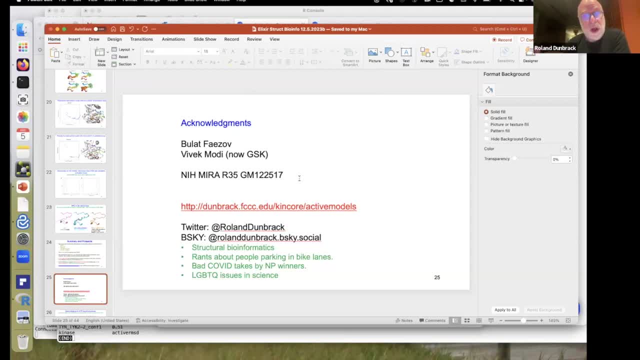 kinase domain but adjacent things that you know really regulate or really interact with the kinase domain. And I think they do all sorts of things. They block the activation loop, they regulate, they interact with other proteins, they get phosphorylated and, you know, fall off. 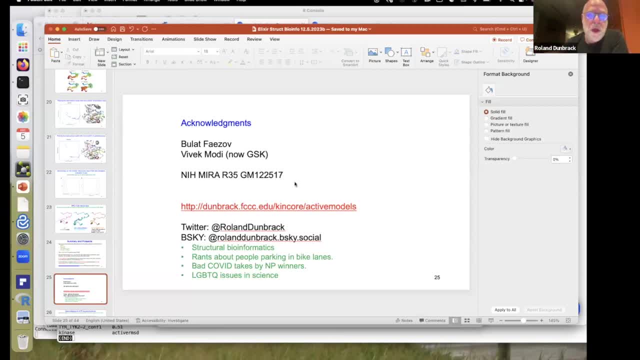 and it might, might make a kinase active or inactive. Um, so yeah, there's lots of interactions of other domains. Um then, for Mark um, is this application to other organisms or structural? um, certainly, all the kinases in, you know, in mammals and and even just higher. 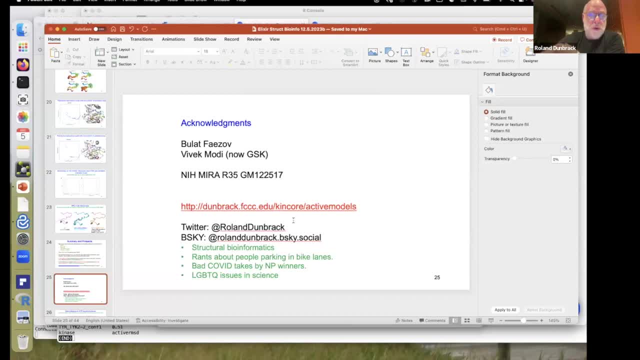 human cariots are very closely related, and this would work just as well for, uh, non-human, uh, non-human kinases, non-human, uh proteins. Okay so, if, uh, if that's all uh, I just 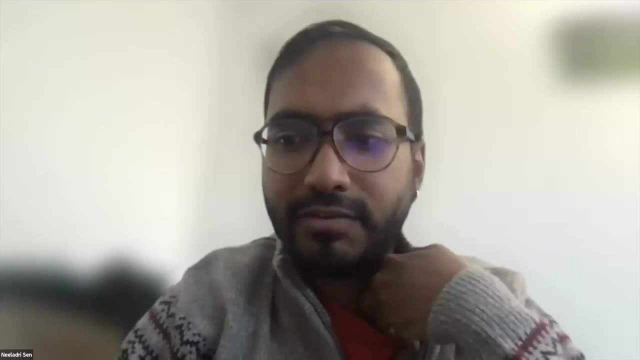 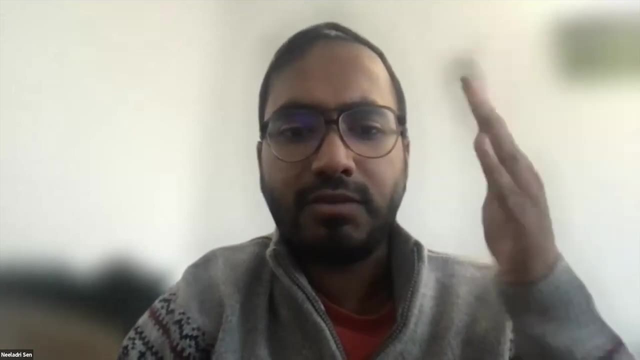 had one last thing. So like you put up like five criteria for the active kinases, Uh, so how important is it to have all five criteria for it to be an actual active kinase? Because, like you showed in the PDV, that if you put different criteria you get different percentages. 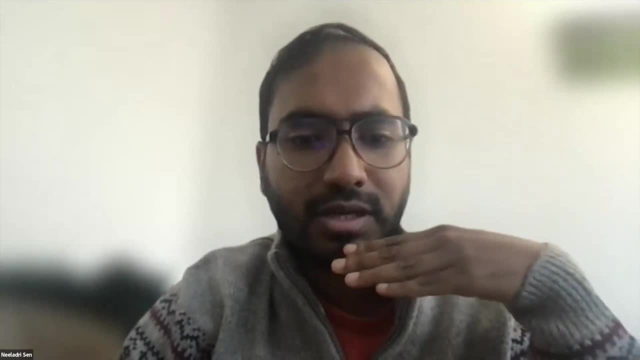 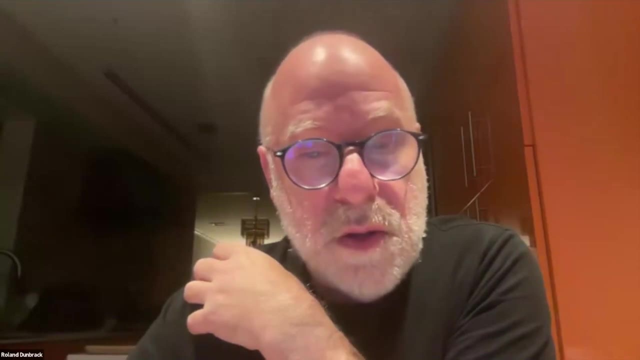 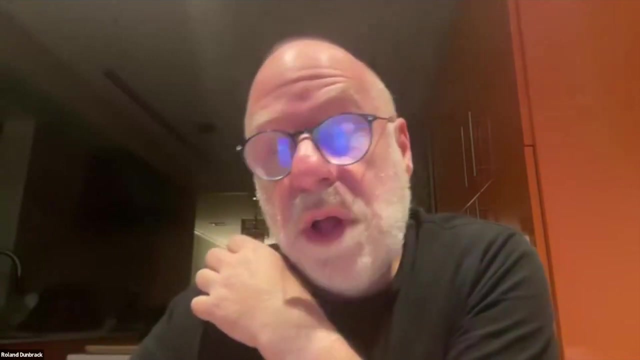 of PDB structures having that criteria. So is I think all five criteria are necessary to get an active kinase That is, to have room for the substrate and ATP and bind it properly. You need to have all five criteria. If we apply all five criteria to structures in the PDB, 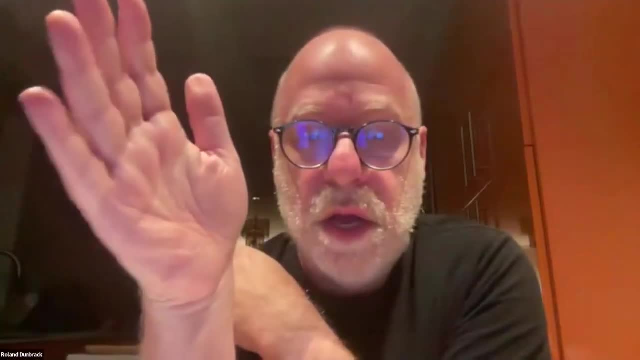 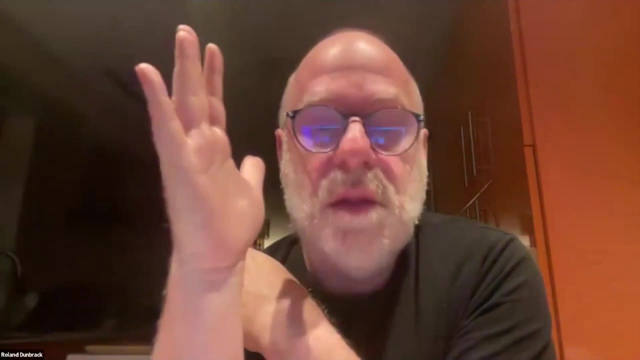 some kinases still have a, some of them. all the structures look absolutely identical and they're all within one angstrom RMSD. Some others have a couple of different populations. I've picked out ones that I think that one looks active and the other one doesn't. 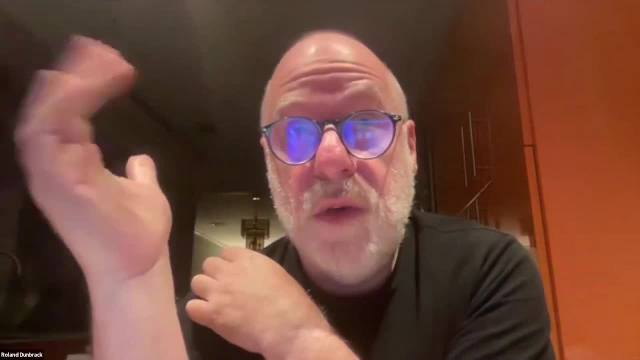 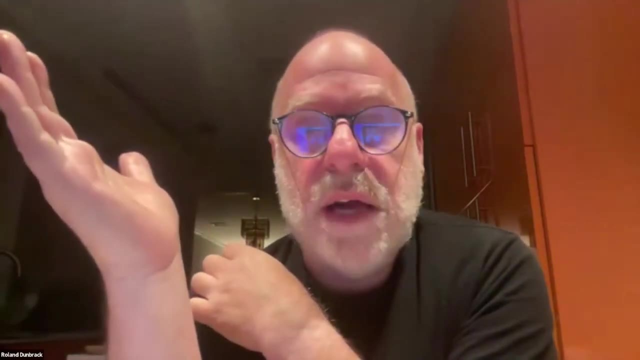 but some of them still have some diversity in the outer parts of the activation loop, even passing all five of our criteria, And I don't know what that means. I don't know if they're all active and they're just, you know, an ensemble of active structures. 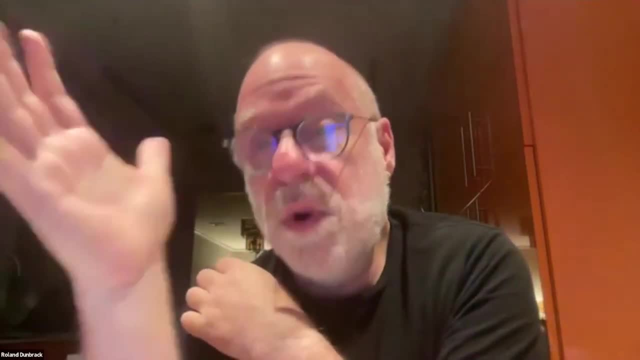 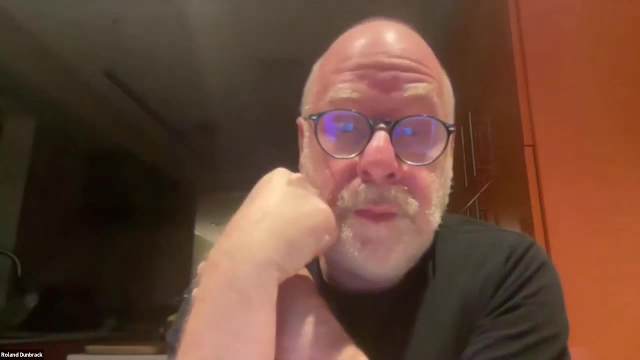 or whether some of them are maybe a little bit less active, and you know they wouldn't bind substrate properly. We don't know that yet, but there is still some diversity left, even after applying our criteria. Okay. Okay, We'd like to thank Roland for his lovely talk. 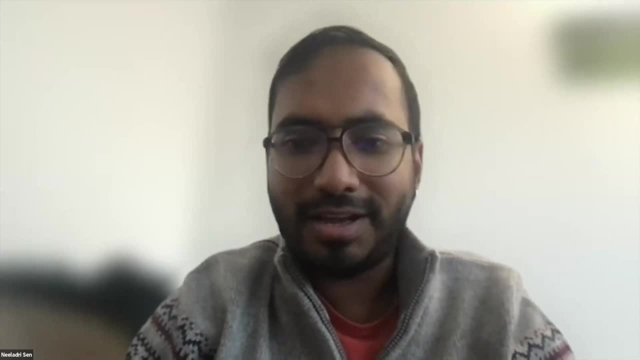 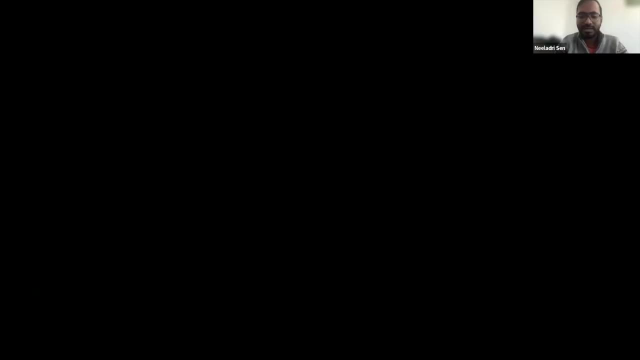 and next we have Michael Stump. Michael, if you could like start the screen share. I'd just give an introduction. like to see if it's So. Michael Stump is a system biology professor at University at Melbourne in the integrative genomics. 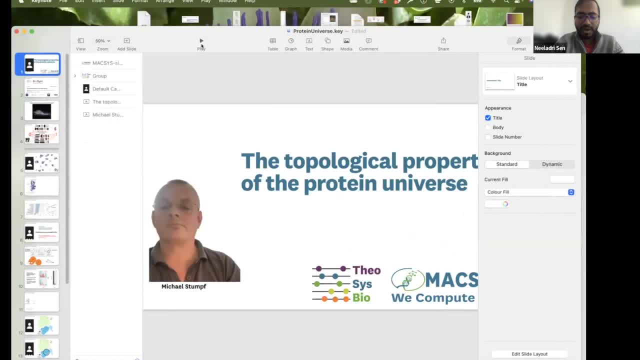 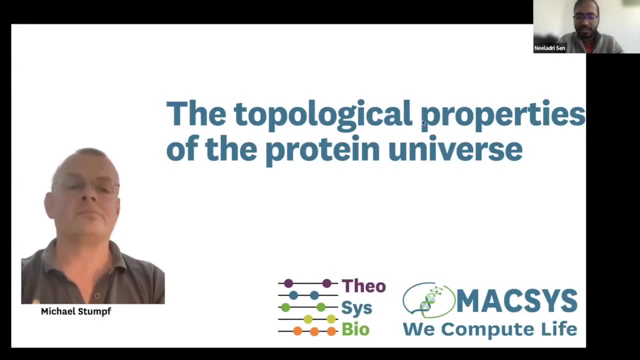 at University of Melbourne. He developed statistical models for biology, molecular networks and send modeling. So he finished his PhD from University of Oxford in physics. After that he joined Imperial College London where he formed his group in 2003.. He has been awarded the Ember Young Investigator Award. 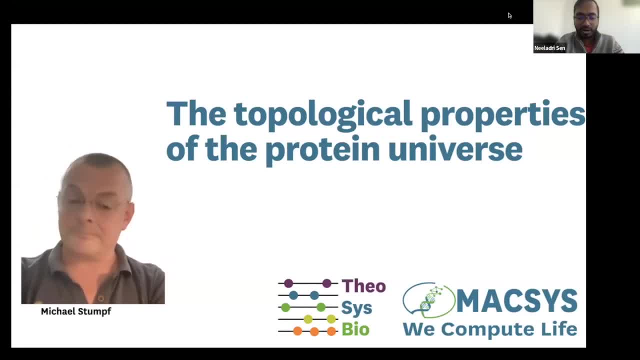 along with a lot of other awards, He moved to Melbourne in 2018.. Today he will be talking about his recent work on topological properties of protein universe. So over to you, Michael. So thank you very much for the invitation. 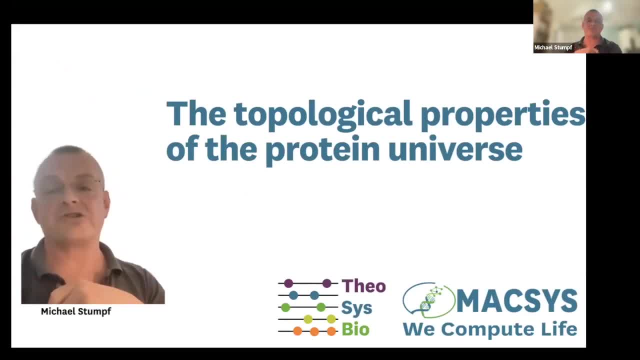 I am not normally a structural biologist, but mostly interested in applying and finding new mathematical methods to describe cellular complexity. but we couldn't resist the fact that, you know this is the temptation to apply some of the tools to this fantastic data resource that AlphaFolder has provided us with. 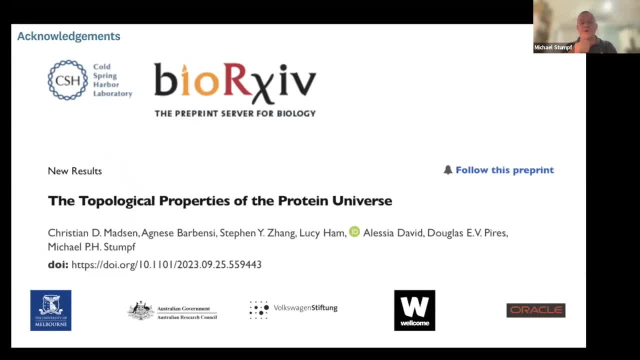 And I'm going to take you to some of our findings here. So the work was carried out by Christian Mattson and Agnesi Babenzi. So Agnesi is now a lecturer in mathematics at the University of Queensland. Christian is a PhD student here in the group. 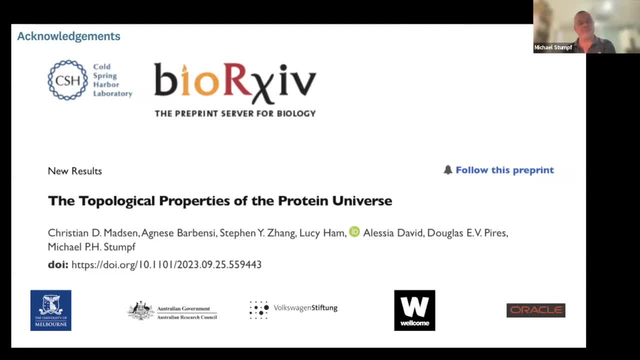 And they have sort of complimented their strengths in bioinformatics and topology respectively. but a whole lot of other people- Stephen Janssen, Lucy Ham, Alessia David at Imperial Douglas Peiris here at Melbourne- contributed And we were lucky enough to get funding. 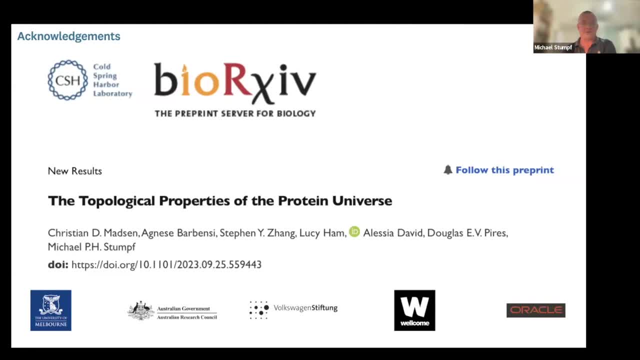 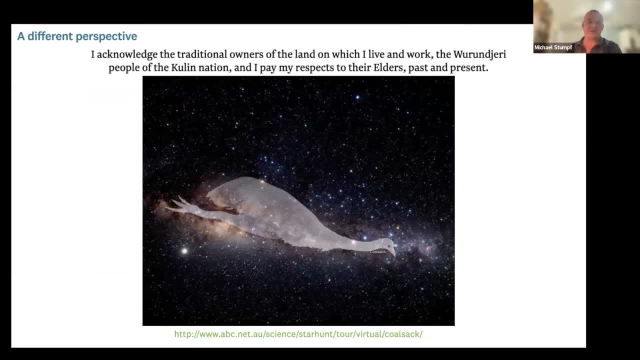 by various funding bodies, including some free compute time and Oracle Research Clouds. I also want to acknowledge, because it's a very good and healthy tradition here, the traditional owners on the land on which I live and work, which, in my case, are the Wurundjeri people. 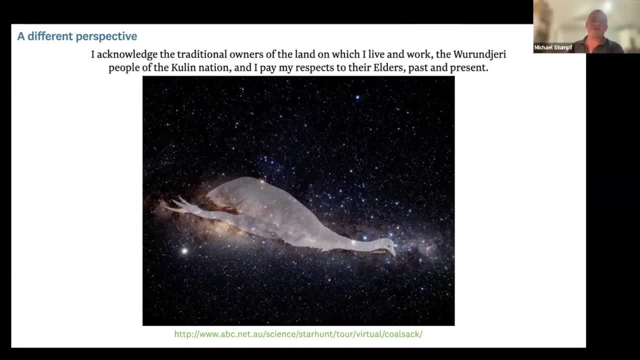 of the Kulin Nation, who were the traditional owners of the land on which we now have Melbourne, And I pay my respect to the elders, past and present, And I also like to thank them for providing this introduction slide, because European and Indian astronomy 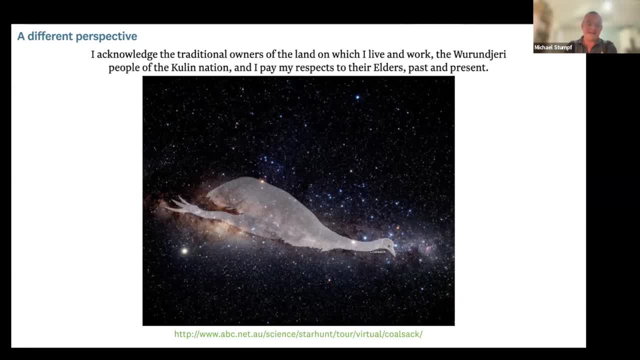 has largely progressed by looking at the stars. First nation Australian Aboriginal astronomy looked at the dark spaces And what we call the Milky Way is sometimes in Aboriginal history referred to as the dark emu, And they looked really at things such as the coal sack. 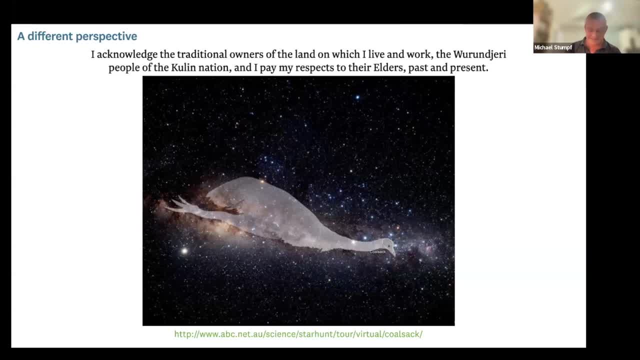 to define the shape, the shape of constellations, And I'm going to do pretty much the same thing today. I really don't care about the structure of proteins, I care about the holes and the voids that they create, And I take this by analogy to pasta. 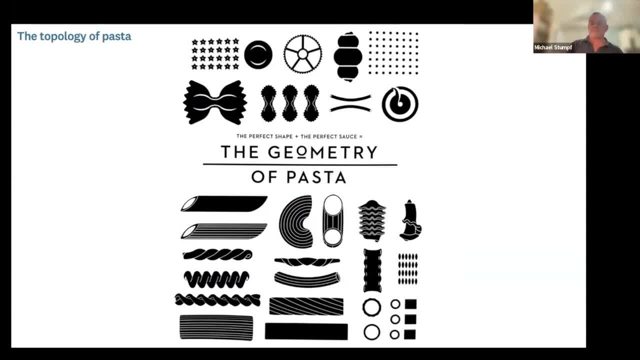 which we all like and know, and it's my favorite illustration of topology, because we're not looking at the geometry of pasta- fantastic book, by the way- but the topology of pasta, And so what we are trying to do is we're now trying to count the number of holes. 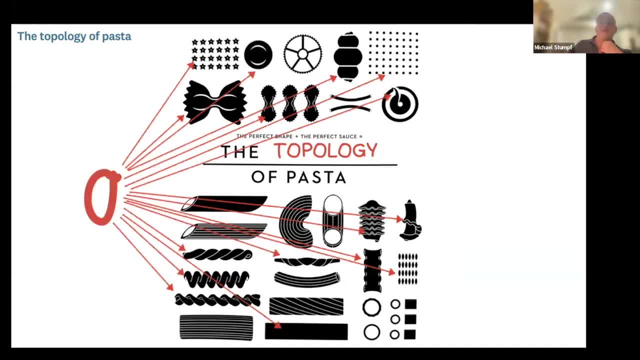 that a structure has And we find that all these different types of pasta here have zero holes. So there's just no way that you would find you would be able to push anything through this pasta without really damaging it, This type of pasta here. 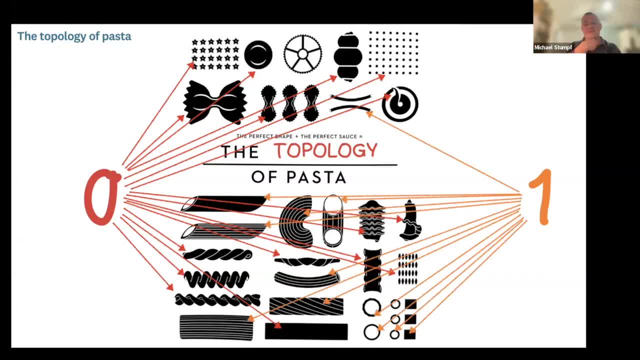 and that includes rigatoni penne, what have you not? they all have at least one hole, So topologically they're equivalent and very, very different from these zero hole pasta types, And that pretty much sorts most of it out. 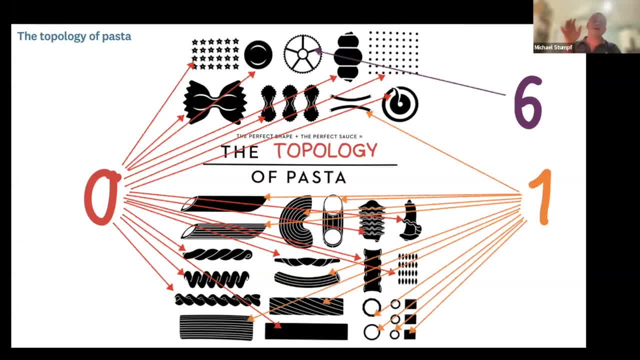 But my son's favorite type of pasta has six holes. So there's no way you can transform this shape here into any of the other shapes without cutting or gluing things together, But through simple twisting, turning and pulling. there's no way to turn any of those topology classes. 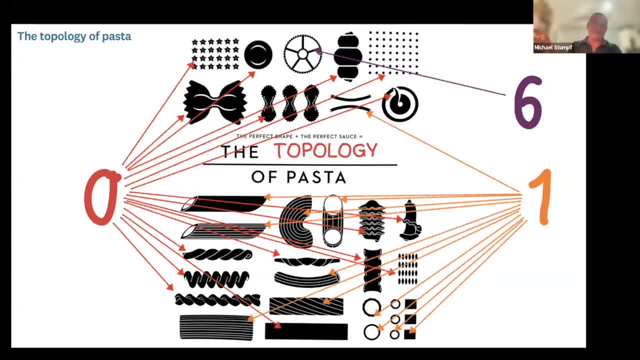 into one another, And so we essentially have a handle on these types of pasta until something like the ravioli comes along, which is a different fish altogether But also relevant for the talk because it has a void, not a single hole, And I will just classify things. 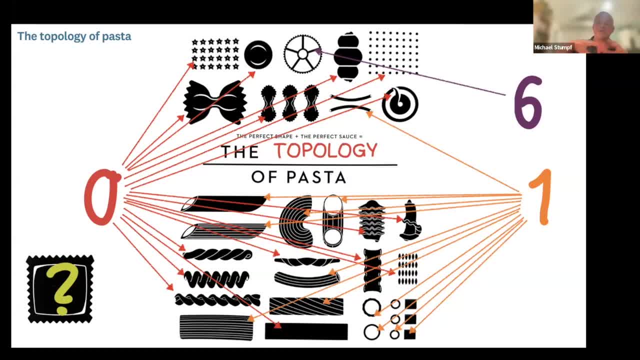 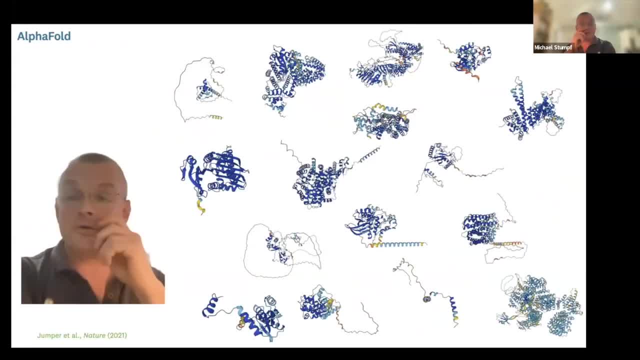 in terms of first-order topological features- loops and second-order topological features- voids that are sort of encompassed in 3D space, And I will take you through our analysis of alpha fold. So this really has changed. how many of my colleagues 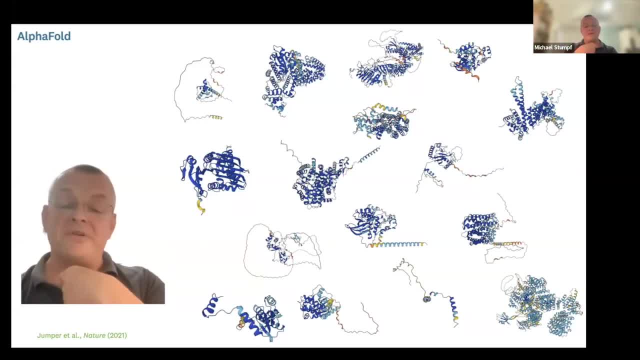 like to do computational biology by reference to this vast data set of 240 meters. It's a million protein structures And for us the interesting question was: how do we make sense? How do we tame this complexity? Can we write a tour guide based on topology? 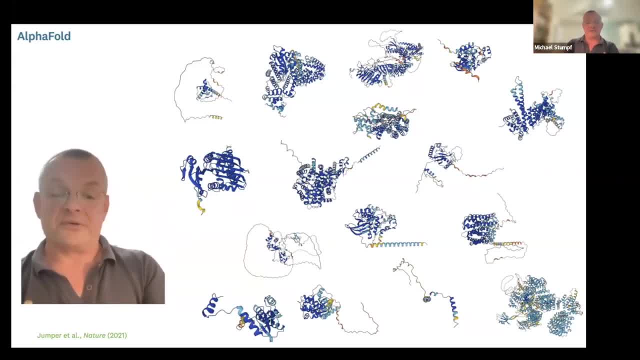 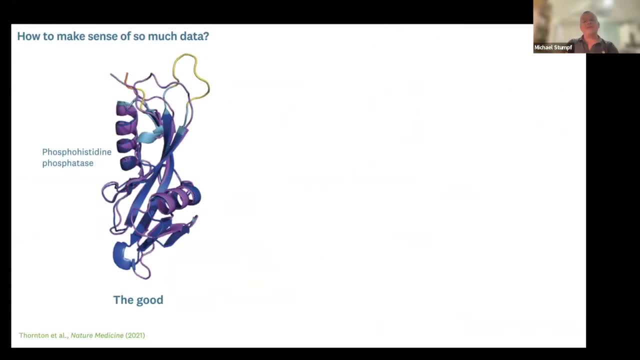 for all these structures that are in this fantastic data resource, And we chose topology as our organizing principle. The question of how to make sense of this data is a profound one, And Janet Thornton and colleagues were one of the first to write a review about how this will. 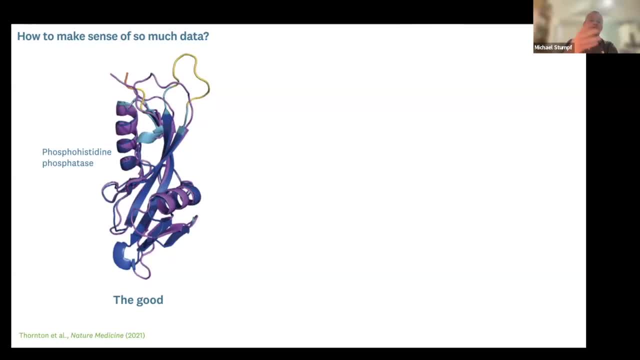 likely transform. We have to be very careful that we don't make sense of much of computational biology And they refer to some structures here- phosphatidine and phosphatase- as the good. Human insulin, the predict structure, is the bad. 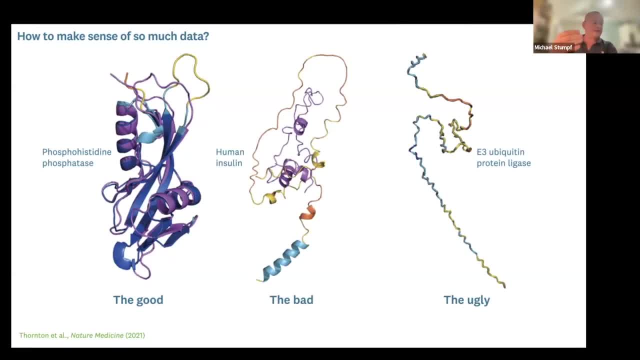 And this E3 ubiquitin protein ligase is the ugly. So if you really go one by one through these 240 million structures, you'll find some that are really conforming to what we know. They conform to what is in PDB by definition. 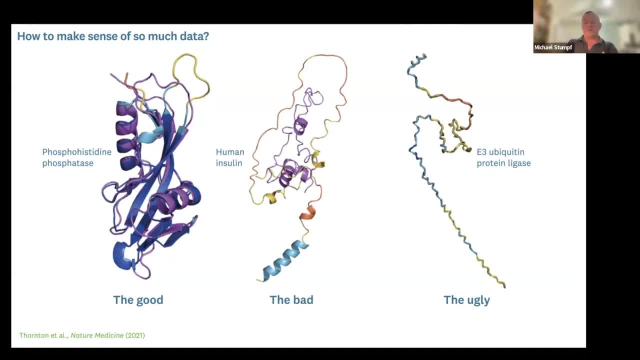 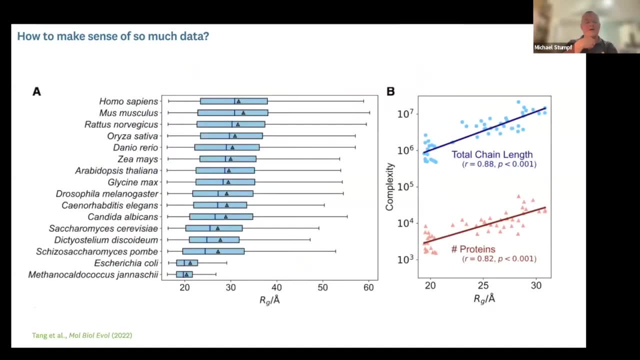 because that was the training input, But others we think that doesn't look like a real protein structure for putting that we like. so you can go through these structures one by one. try to make some sense. other colleagues, so tang et al, as from kineko, kaneco's group, have tried to make sense of 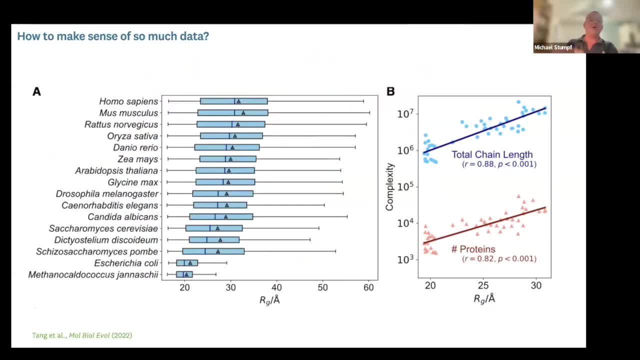 the structure in a sort of organism level. try to see if organismic complexity corresponds to some simple measure, for example here on the left hand side to the radius of gyration for roughly equally long proteins, and they looked at protein chain lengths and complexity as captured by the radius. 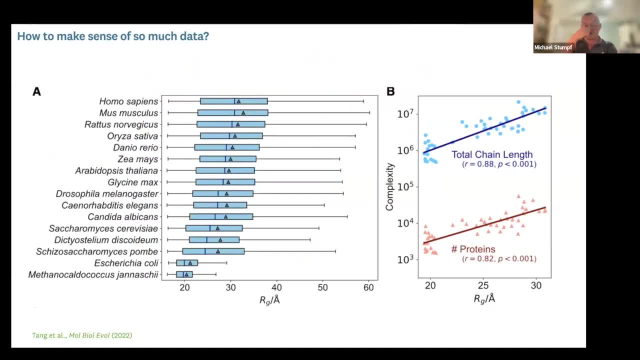 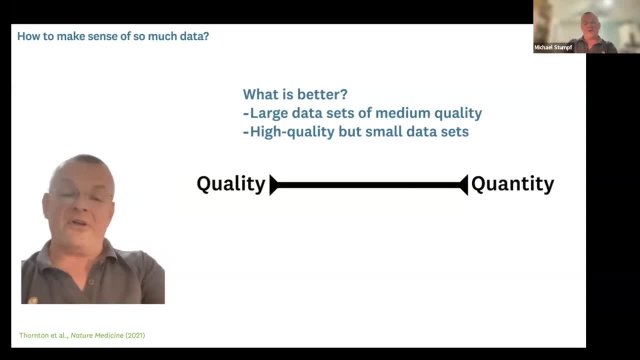 of gyration for them, for these protein structure predictions. so we are taking this other type of approach and it's largely based on on sort of it's a quasi-philosophical question: what is better? do you want to have large amounts of data with medium or acceptable quality, or do you want to? 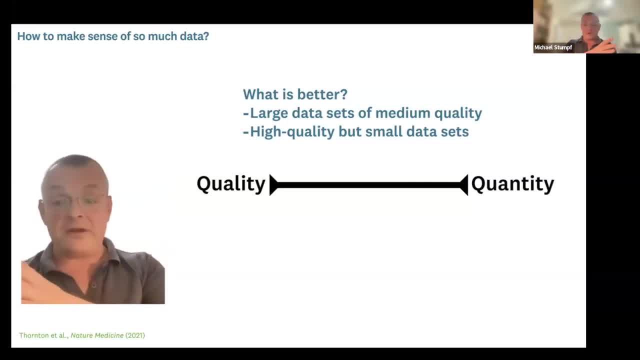 look at high quality data but very small data sets. so this trade-off between the quantity and the quality that we want to look of is something that concerns us a lot in our day-to-day work. but we can start by agreeing that our analysis should not really destroy the signal that's in the data, and that's what we try. 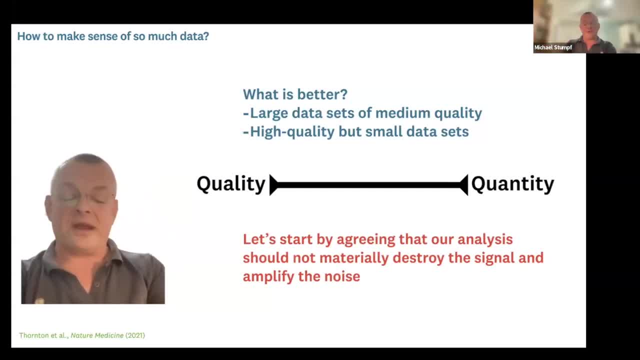 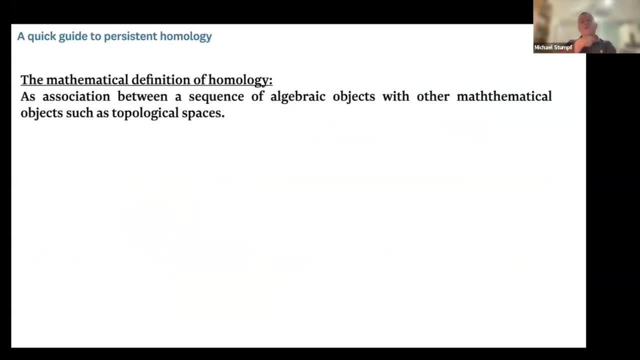 to set out to do by taking this very coarse grain perspective that the topological lens affords us with. I'm going to use a concept called homology and the different types of homology. that we use a concept called homology and the difference in the different types of homology. that we use a concept called homology and the different. 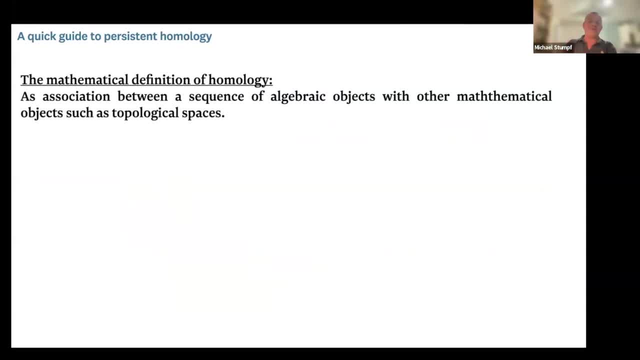 The definition of homology in mathematics is very different from the one that you all will be familiar with. So the mathematical definition of homology is an association between a sequence of algebraic objects with something that is a topological space. In more normal words, it's a relationship between something discrete and something continuous. 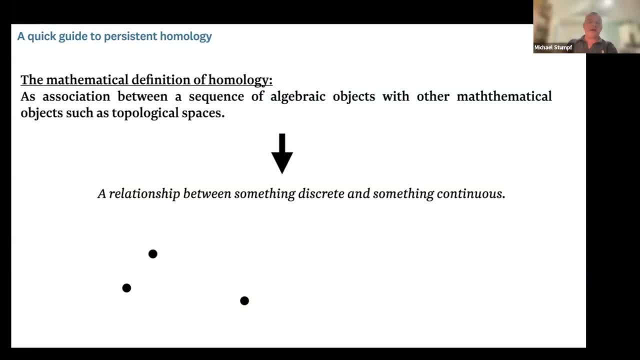 And if I have three points in space, they are some distance apart and I would like to learn some relationship from them. I can do this in a number of ways. What we are using is called persistent homology, So we are slowly growing a radius around each of those points until the circles start to overlap. 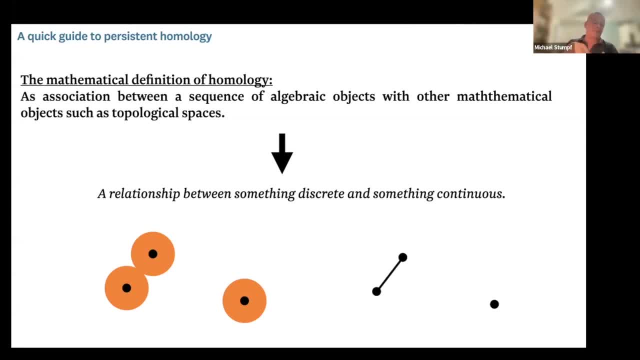 If that happens, we say from this radius onward we have an interaction between the two dots on the left, On the left hand side, we let the circles grow further until we have another touching set of circles And we now know that the node here and here interact. 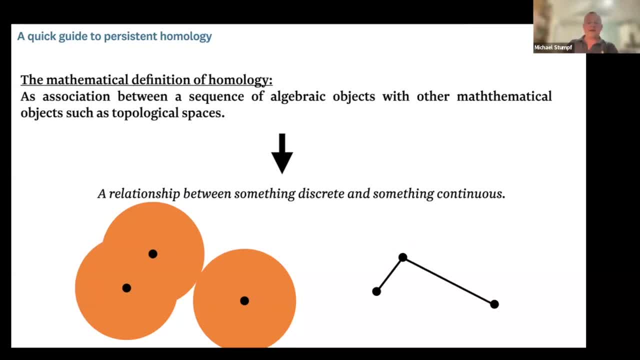 So we draw an edge between them here And we can go further and grow this further until we now have all three circles overlapping And we can draw the final third edge between them And we can look at either three edges Or, if you just try to go further, 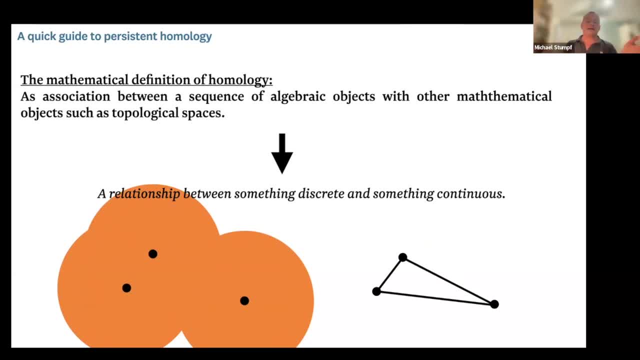 you can go deeper into the mathematical toolset. We can now treat this as what's called a simplex That has three sides to it, And so we are using these types of relationships that link on the left hand side, something in real space with a graph structure. 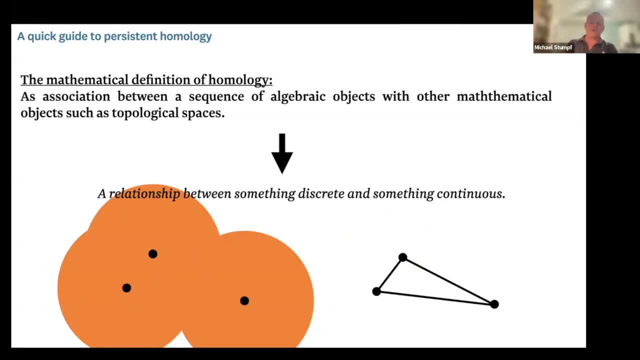 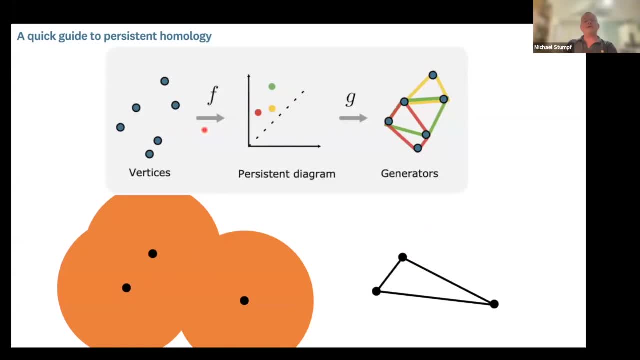 In our case, we use a hypergraph structure in discrete space. So this is what we use when we talk about homology. So we are taking now vertices in space. We plot here. when do we first see such a structure? When do the structure becomes obliterated by a higher order dimensional? so simplex. 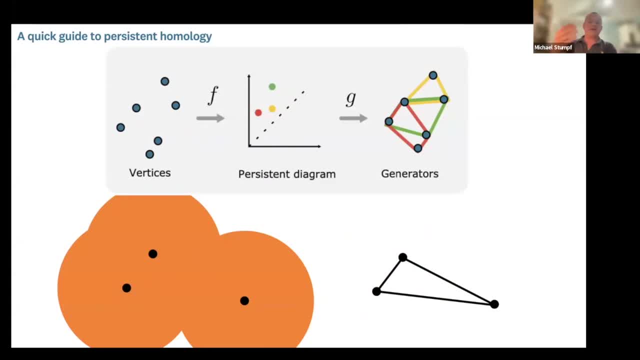 And we draw this persistent diagram, And from this persistent diagram we are trying to influence, identify those structures, substructures that are most likely to drive the overall structure that we see in the data here. So we're going from something very coarse grained to something more mathematically amenable. 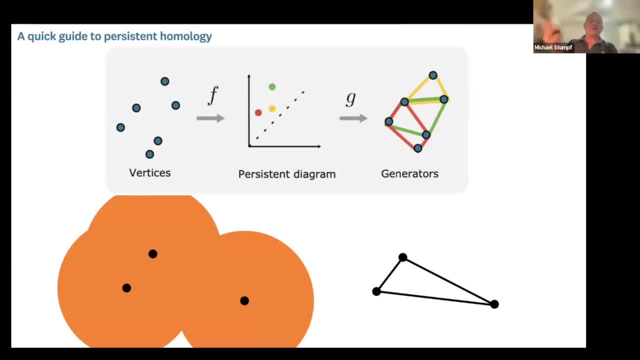 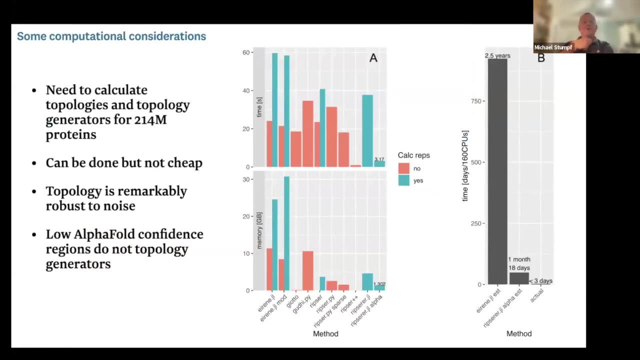 And then we try to see what determines the overall structure. But the advantage that we have is we don't have to pose any sort of outside constraints on how we define these structures, So we just really let the data guide us. So we have to go through this process some 214 million times. 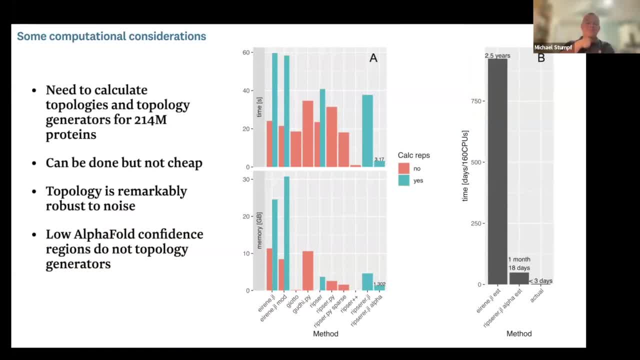 And that is doable, but it's not computationally cheap. The advantage that our approach has- and in the preprint we go to some length trying to make this robust- is that topology is really robust to noise. So, in particular, those regions in alpha fold that correspond to low confidence regions never contain the types of things that we would call topology generators. 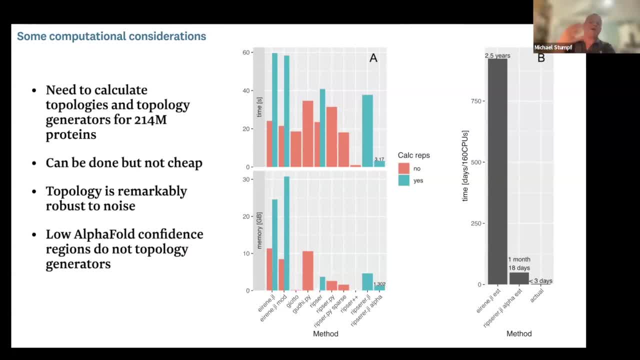 So they're topologically and in our view therefore quite boring, Because we have to do this so a lot. We spend an awful lot of time benchmarking different algorithms, making sure we have the fastest possible approach, and we can do this with finite amounts of memory. 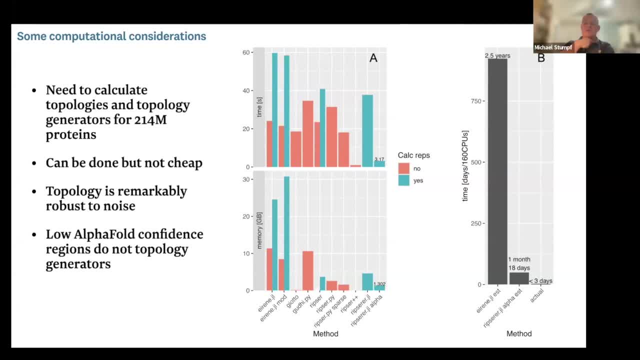 And what initially struck us as a two and a half year job with 160 CPUs, in the end, through optimization using Julia rather than Python or other sort of languages, made it possible to do this in less than three days Plus, on top of that, we did some robustness analysis. 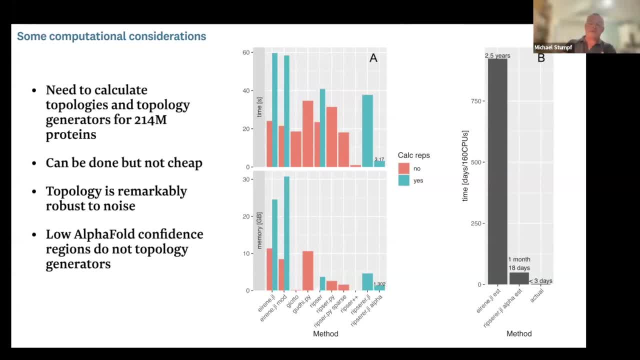 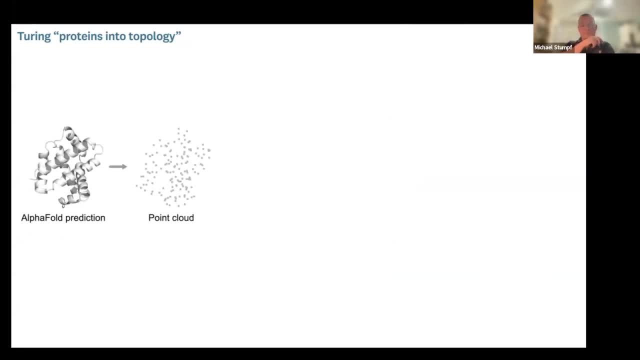 So this was really possible because of his determination to make this fit into very comfortable into the first year of his PhD. So what we are doing in practice is we take the alpha fold predictions, We use the backbone carbon alpha atom and we place a point in 3D space to create a point cloud. so this is the translation from the alpha fold prediction into point cloud. 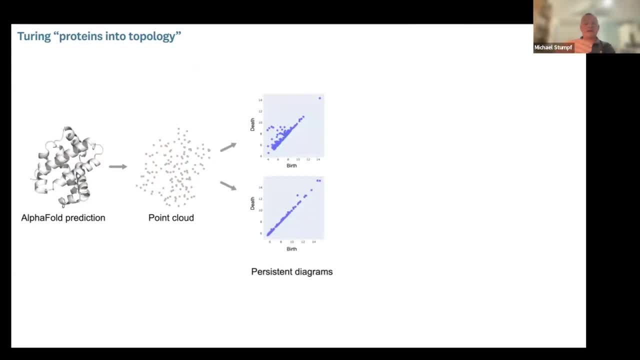 So this is the translation from the alpha fold prediction into point cloud. So this is the translation from the alpha fold prediction into point cloud. We calculate the persistence diagram that corresponds to these structures And we then map these persistent features back onto the protein structure and identify those sequences though those structural elements that really drive the 3D structure. we look at loops, those will be the holes and pasta, and we 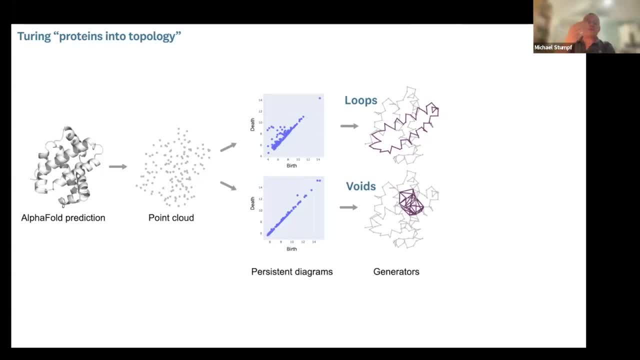 look at the voids, which would be so confined points in three dimensional space, like the right and left sides, like the ravioli that I showed before, And then for each point in the protein we can calculate something: the topological influence scores. that is a measure for how often a given residue 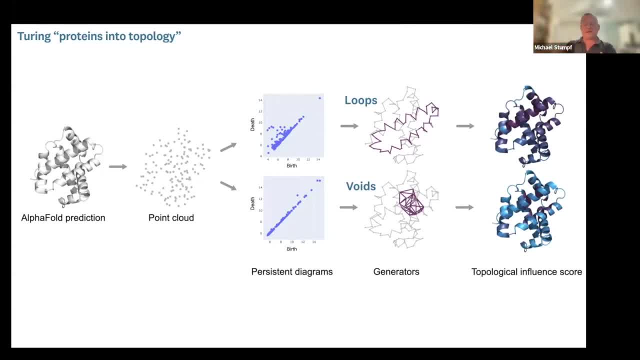 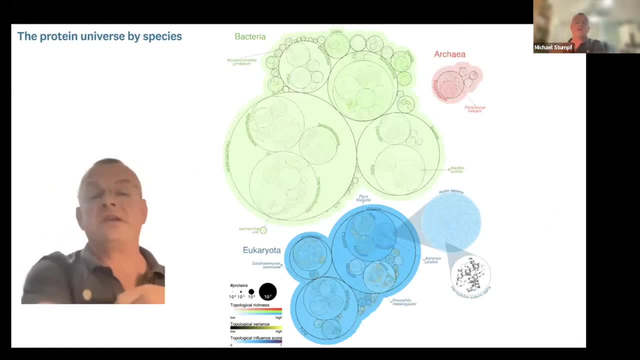 is involved in a feature that drives the overall topology of these proteins, And we do this for all 240 million proteins Here. Christian and Agnese have provided a sort of overview over the different kingdoms that we had. We look at Biteria, Archaea and Eukaryota. We find we were 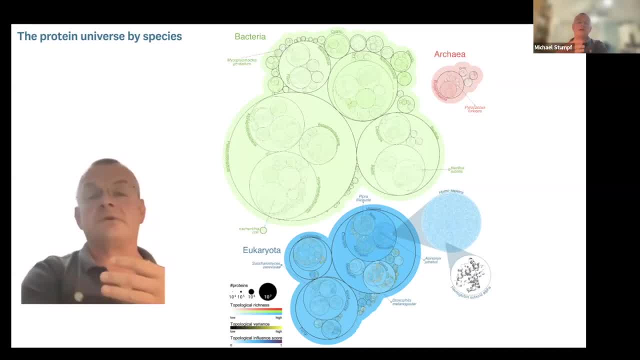 particularly interested at a couple of model organisms that the group is looking at anyway. so E coli, Abyssalosatellis, of course, Cerevisia and humans. We looked and we tried to identify what type of species in the alpha fold prediction are diverse or rich in terms of topology. 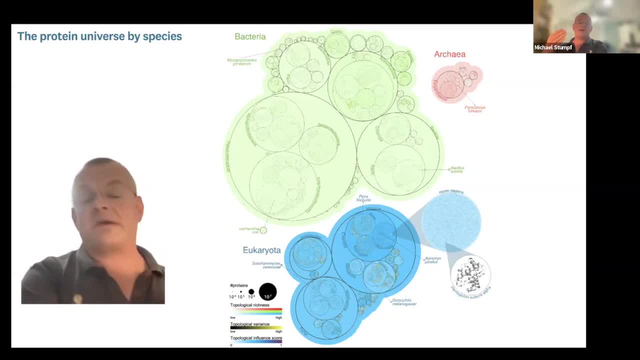 And the richest species- and I wouldn't really read too much into this- is down here. That's the cheetah. So there's no particular reason why this should be very rich. But we then looked in more detail at what we find here. 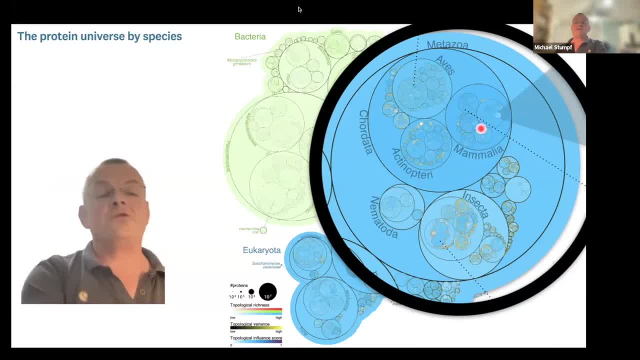 in the in among the mammals, the humans, And we find humans and the color code is here, but it's much, much clearer in the paper, in the preprint. Humans are actually topologically not as rich as many of the other mammals And that suggests that we have. 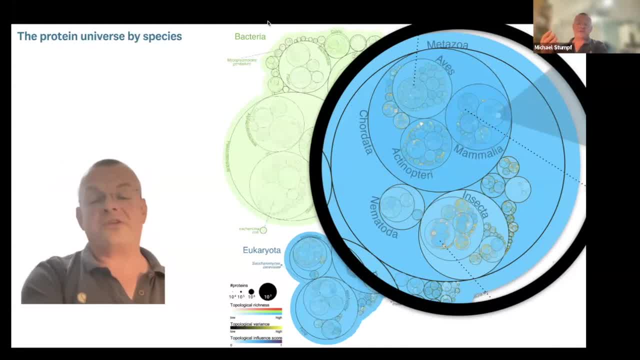 different levels of organization that give complexity to humans over other organisms. But it's for us. it was only a starting point, trying to see can we learn something from this. But overall it starts to give an idea that the topological complexity alone does not drive. 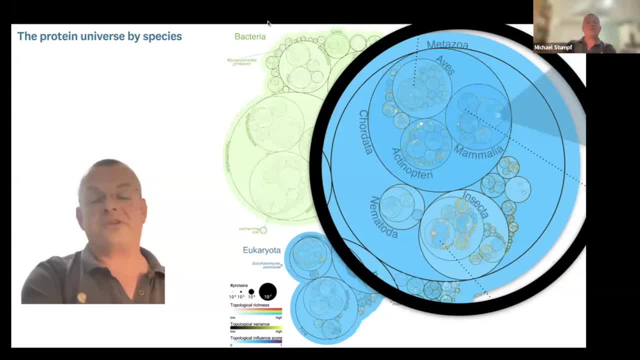 the complexity of an organism in the sort of conventions. Oh so can you see it now again? Sorry, Sorry, I'm not quite sure what happened there. So the mammals are, the humans are one of the less diverse species, cheetah by far the most diverse species that we 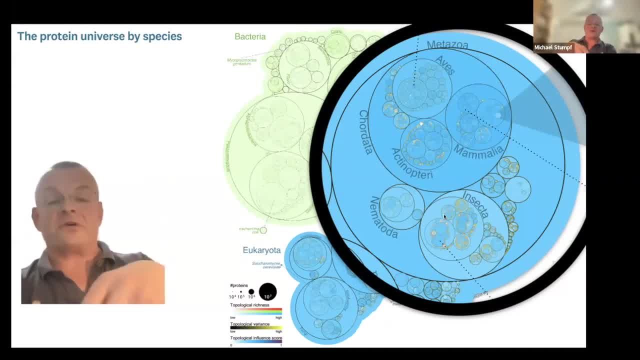 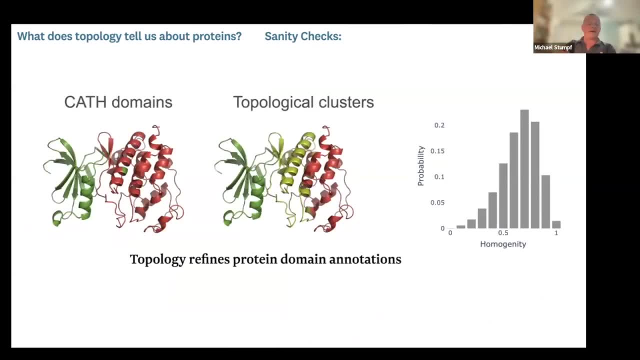 have in our data set among the mammals. But there we go. So now we try to see what else do we find in our data And we perform a couple of sanity checks. The first thing we did is try to see if topological features that we identify are linked to something which structural biologists have. 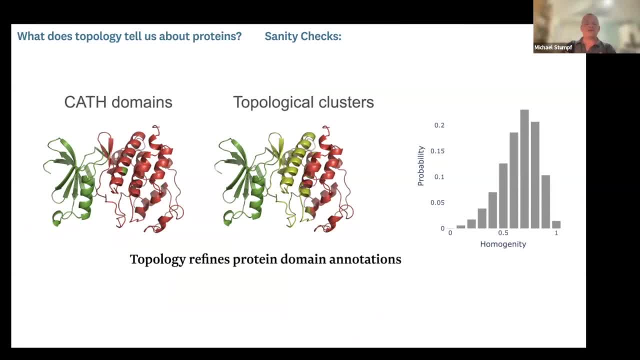 studied for a long time particular cath domains, other domain definitions, And we find that by and large the clusters that topological measures assign correspond very nicely with domains in cath and other databases but potentially find a little bit So. fairly frequently you find that a 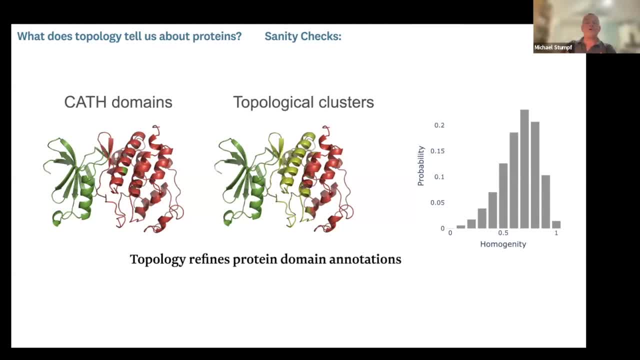 traditional cath domain would correspond to a cluster that has topological features that are much more than one topological cluster, But in a way which, for example highlighted here, is not outrageous. So you wouldn't be surprised if somebody were to tell you this, And we can. 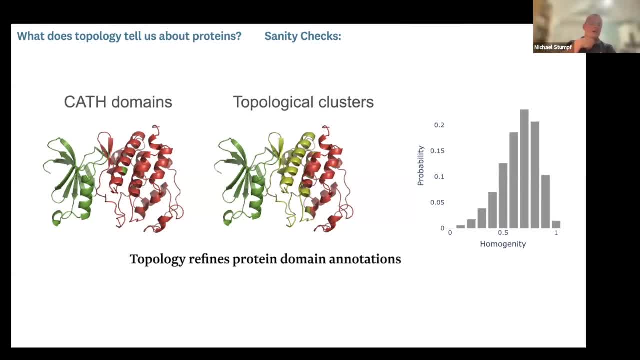 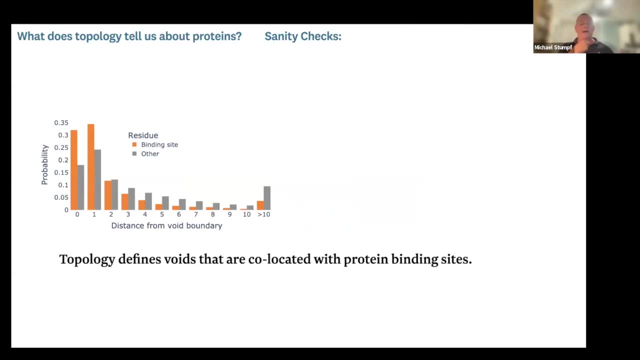 quantify this by the homogeneity score, But more or less we find very good agreement between traditional domain annotations and the domains that are purely defined in terms of topological features. What we also found when looking at the mechanism in catalytic site atlas is that topology defines voids in the protein structure that are co-located with active. 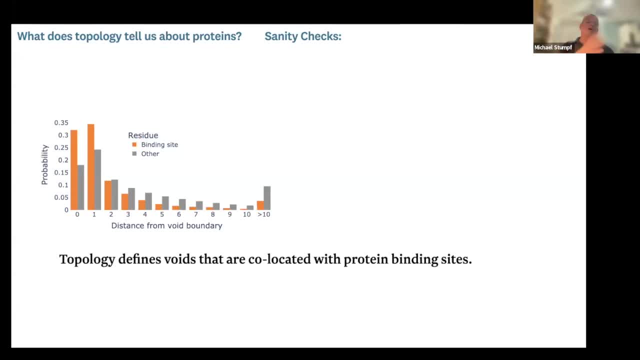 sites or with protein binding sites, So they tend to be closer to the boundary of a void than you would expect to occur by chance. So this is something which we also think is reflecting some baseline sanity of our approach, And we found that the topology of alpha-fold proteins 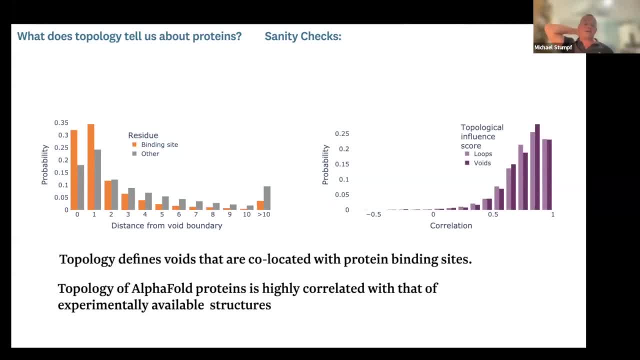 is highly correlated with that of experimentally available structures. Again, this is not so surprising, because those structures clearly fed into the alpha-fold algorithm. but by and large, this means that we can now focus on the analysis of alpha-fold and not have to always explicitly 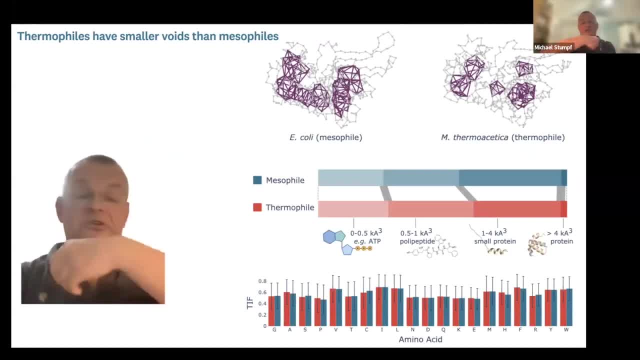 go back to PDP or other structures For our purposes. Then we start to think about what other aspects of biology might be interesting And we hit upon two facts that we found were reasonably unexpected and news and for us, new. And the first one was we looked at the topological features in mesophiles. 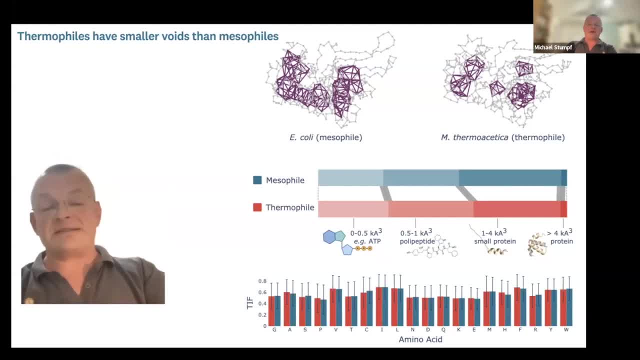 such as E coli and in thermophiles, trying to see is there a difference in the structure and the size and other characteristics of the voids that we have in these organisms And we find for clearly defined, unambiguous orthologs that in the majority of cases smaller voids are over. 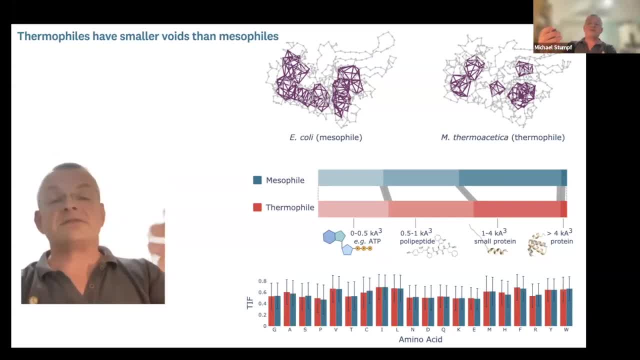 represented among the thermophiles compared to mesophiles. So you see here that very small voids are more common in mesophiles, in thermophiles, than mesophiles. Larger voids are more common in mesophiles than in thermophiles, And that is something which we found. 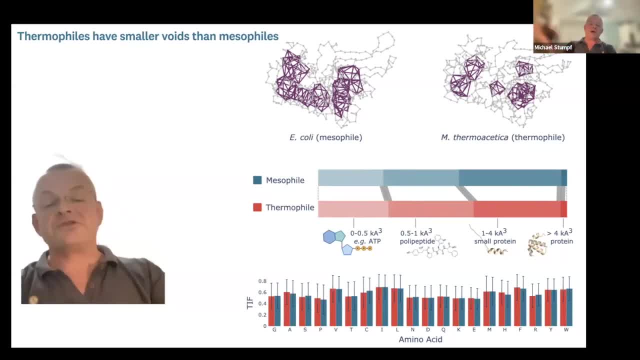 across all the molecules that we looked at, but also across individual, in each individual enzyme EC classes we try to see. do we see a consistent pattern in different EC categories? And we also were able to rule out that the differences in void size are caused by the 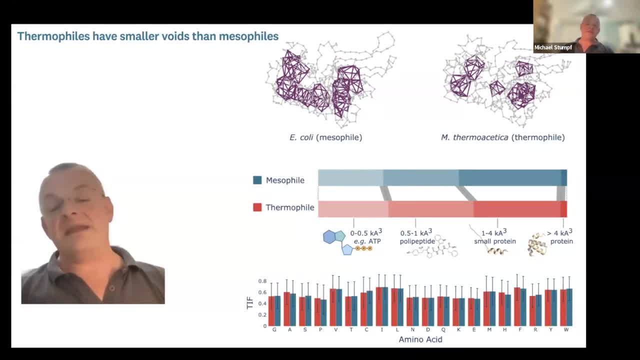 volume of different amino acids. So you see that in these voids they're pretty much distributed as equally as you would expect to occur under these circumstances. So this is something which we found, Michael, sorry, Hello, We can't hear you. 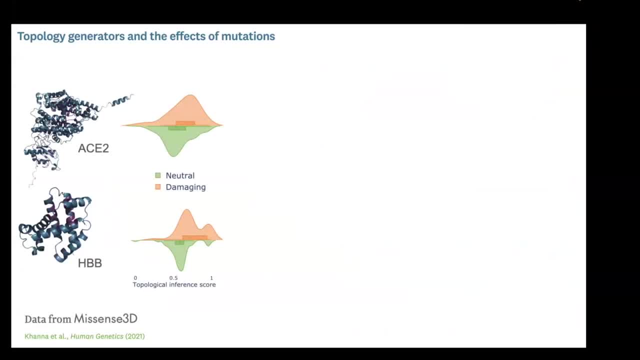 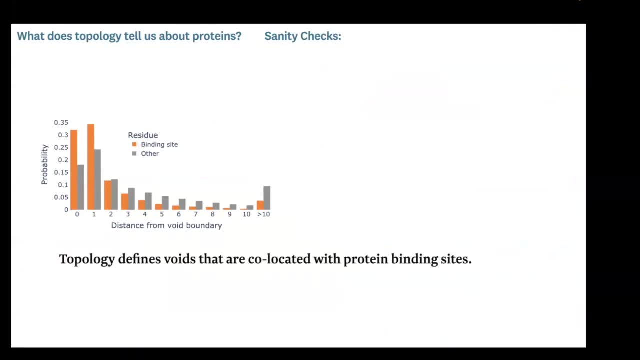 Oh, Now it's okay. Can you hear me now? Yeah, yeah, yeah, So when did I drop out? When you were talking about the void sizes depending on the amino acids? Okay, So, okay, That's all. 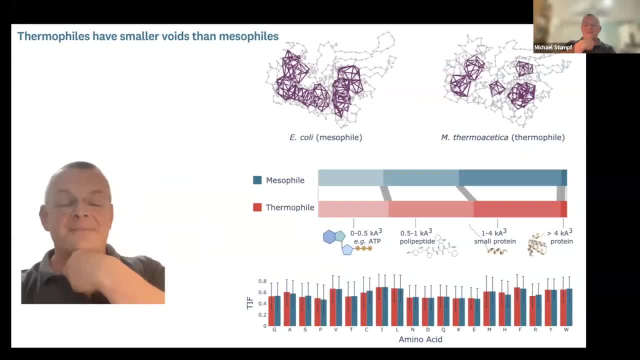 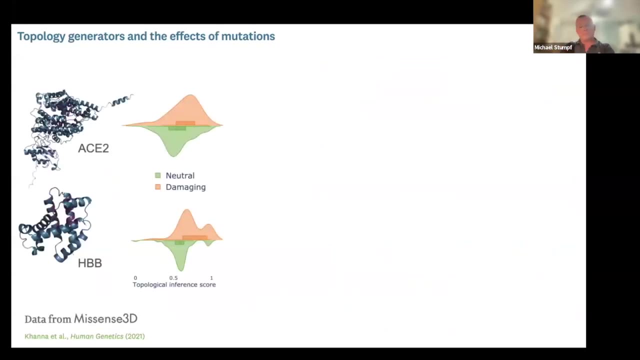 If you haven't missed that much, then that's good. So we find that the amino acids are equally represented among in the voids in thermophiles and mesophiles. there's no secular difference in the amino acid composition, something we're very keen to rule out. 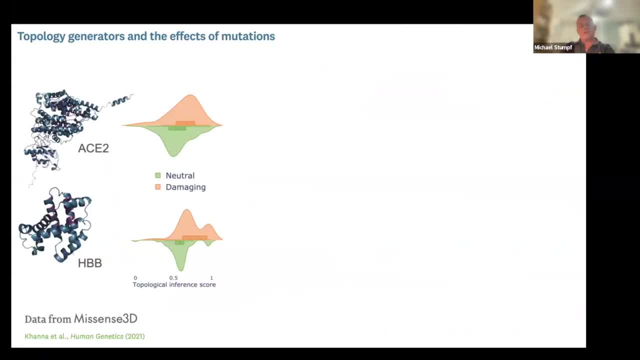 The other thing that we were looking at- and that is one of the few situations where so our first guess was borne out by more detailed statistic analysis- was trying to see if mutations, where we have a good idea, if they're neutral, or damaging if they. 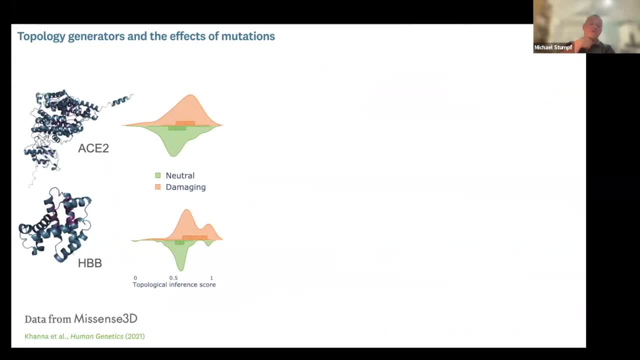 correspond to topological features. Our first two examples were ACE2 and HPB and we tried to see: are there what's the topological inference score, some measure of the topological importance for mutations that are neutral versus mutations that are damaging? and we found in both our first examples, 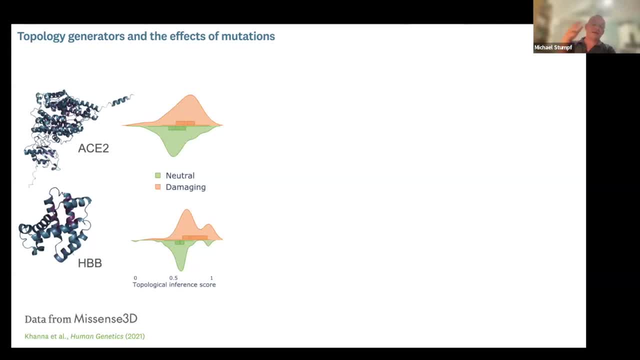 that the the spectrum of the damaging mutations is shifted towards higher topological influence scores compared to neutral, and we found the same thing for both proteins. What surprised me and caused me a sort of slightly sleepless night while I was waiting for the results is that also is the case if you look at all the proteins that are in. 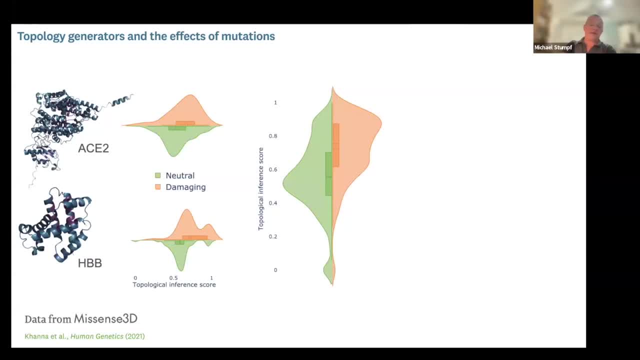 this database, missense3D, that was created by Alessia and David at Imperial College and my former colleague Mike Sternberg. And so you really find that the topological, the topological influence score, our measure of how important in a topological sense, a 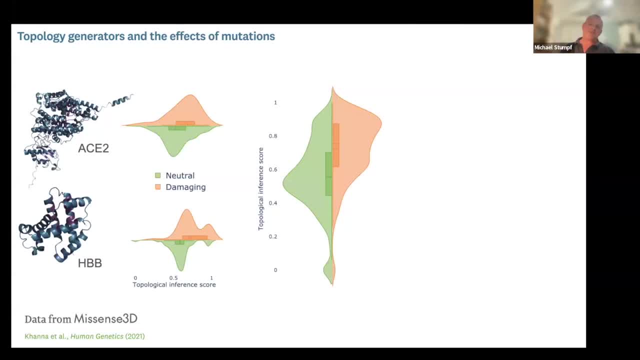 residue is does seem to chime with baseline intuition that you have that those sites that are important in shaping the topology or the structure of the protein measured by topology, are enriched for mutations that have some deleterious effect or some structural effect. And we looked at them separately and in combination and we're going through this. 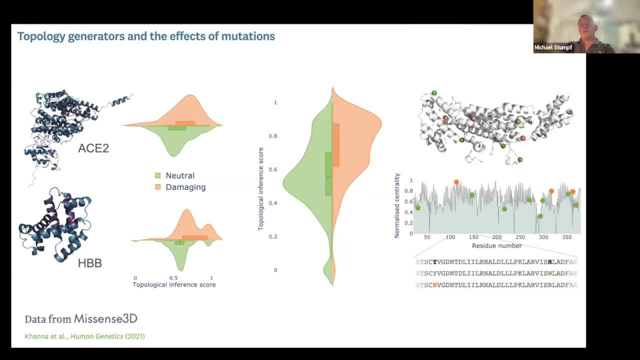 in some detail in the paper, And so what you see is here that if you look at a measure of the importance- in this case we use a centrality in the hypergraph that represents our topological analysis- is we find that damaging mutations are associated with higher topological centrality. 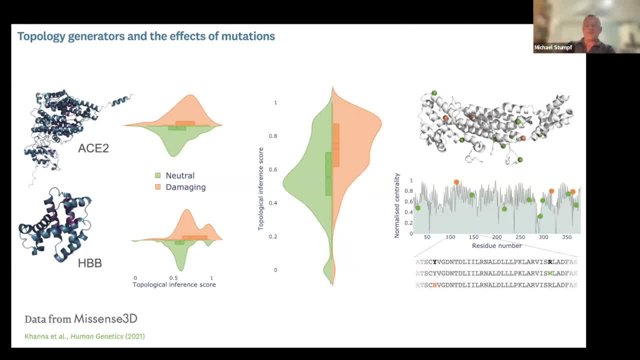 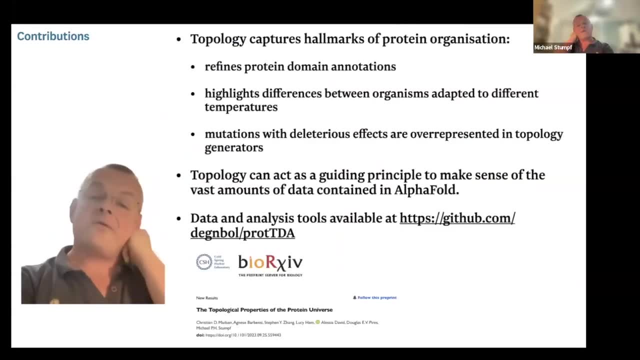 compared to the green mutations, which are neutral to all intents and purposes, and what we know, So what we're fairly confident about now, is that topology is able to capture hallmarks of protein organization that is independent of the sequence. So we look at the topology without any 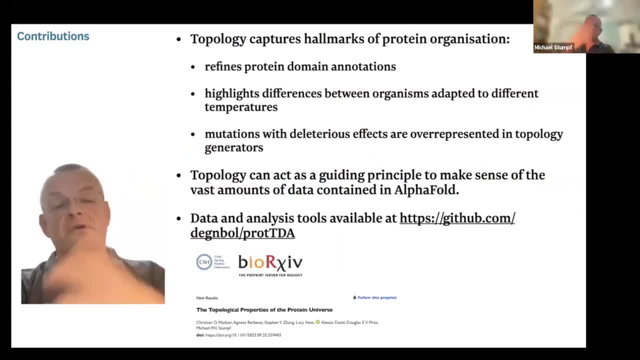 reference to the topological analysis. So we look at the topology without any reference to the topological analysis. So we look at the topology without any reference to the topological analysis. the primary sequence: we only looked at sequence later on if you were to try to get some sort of 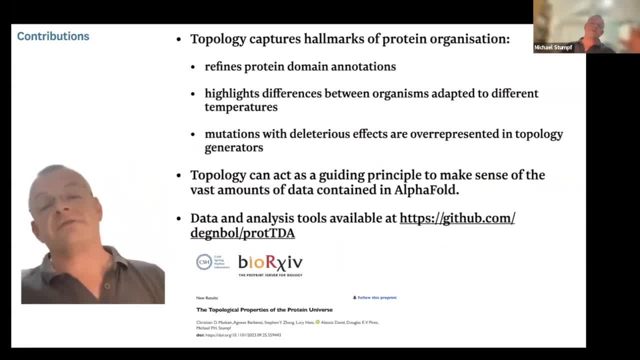 statistical insight into, into overall patterns, and so this is measured by, in our mind, by a few things. first of all, we find there is a nice correlation with protein domain annotations and the position of active sites, catalytic sites, binding sites, as tabulated in in high quality. 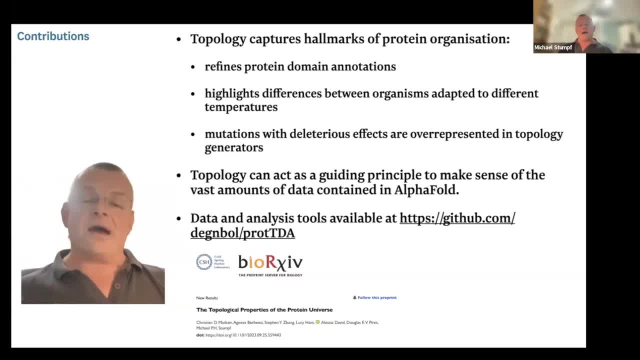 data sets to our sort of delight. we found that topology shows some secular differences between organisms that are adapted to different temperatures. so, in in the sense that a protein, an organism that prefers to live at higher temperature, tends to be less determined by large voids, it seems to be sticking slightly more closer together the void, the internal voids. 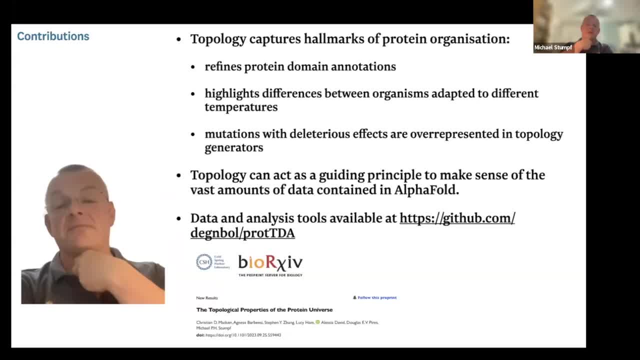 are smaller by some significant margin compared to the mesophilic orthologs, and mutations with deleterious and or structural effects are over represented in these topology generators that we can identify using this approach. so what we set out to do is we're really trying to see if topology makes sense. 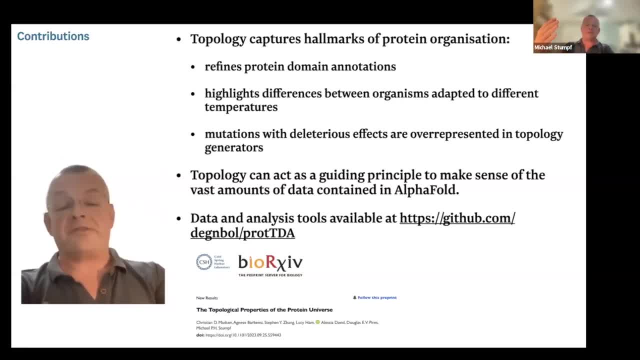 and topology is really, until very recently was a branch of pure mathematics- not at all applied mathematics- but it has some gain. subtraction in topological data, as for example, but also with the approaches that we've made available, can be applied to some structured data. it includes a 3d structured data of proteins or or other long molecules and 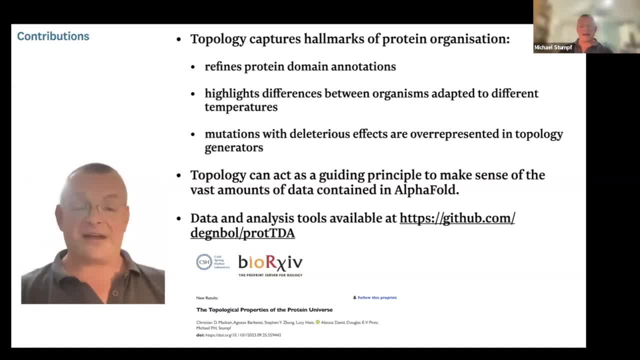 we would argue now. so my group and i would argue that topology can act as a guiding principle or as a tour guide to make sense of certain sections of this vast amount of data that is contained alpha fold. so if you want to look and check the data and the analysis tools, please feel. 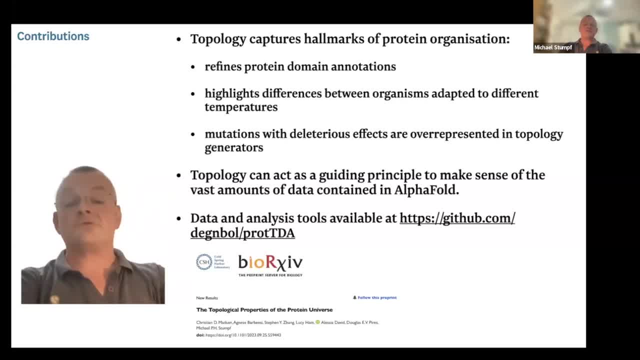 free to look at at this github website. it's also referenced in the paper, the papers on bio archive, and we would love to hear from people with uh problems, criticisms or suggestions that they have for this paper, for this methodology, and i want to conclude with this, so we already have a few una there. so, yeah, if you look at it, uh, have you tested whether, how well 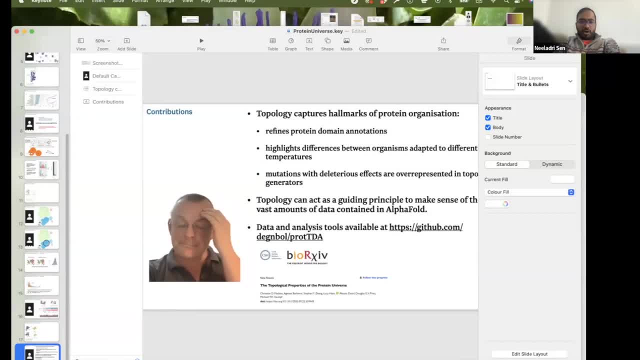 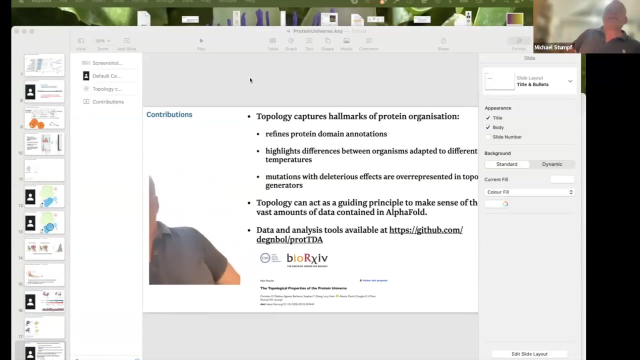 our organisms described in alpha fold, influence your organism specific results, example via busco. and so let me, let me have a look. if i can see this, i have to find my. so yes, we've tested some of that. it's um. it was really hard to identify comparable orthologs. we had to filter quite hard. 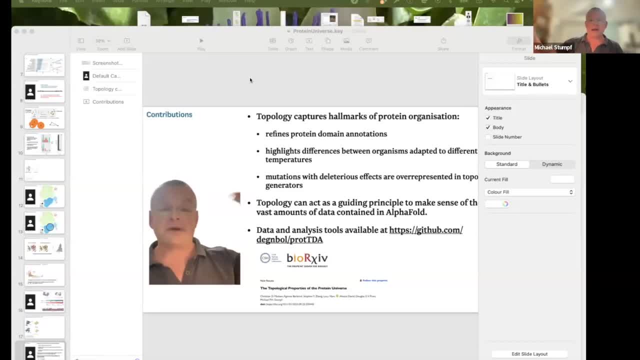 to make sure that we don't introduce some bias by looking at Penrith's longer proteins in one circumstance compared to others. So we found, once we've done that filtering, there was no organism specific effect that we could identify beyond the ones that we were interested in when we looked at. 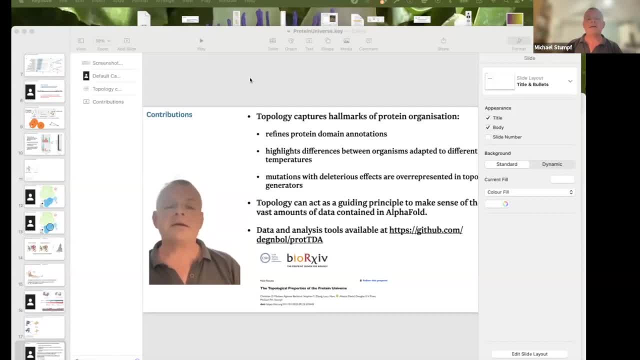 at mesophile versus thermophile. Yes, I hope that answered the question. The next by Vasilis is: that's a very good point. So could the diversity in chronological complexity be attributed to artifacts caused by lower quality of gene annotations? gene prediction in non-model species. 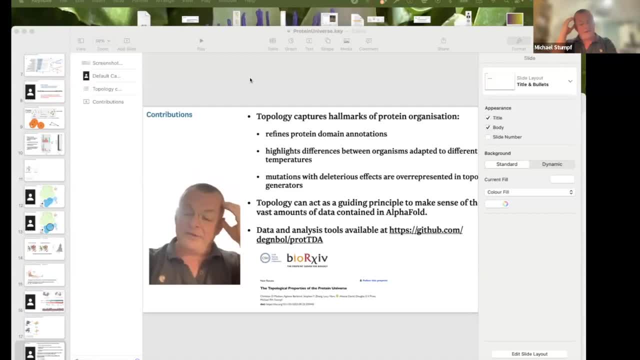 We write about this a lot and we looked a lot at proteins. So we looked at, we filtered proteins by different ways, So we looked at the reliability or the confidence scores that AlphaFold assigns and we found that all the regions that are not assigned a structure that is at all 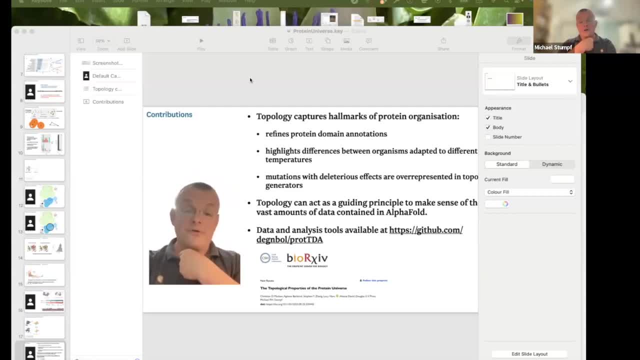 reliable, never generate a topology generator. So that would be stuff that is missed entirely from AlphaFold, but it's so. if AlphaFold is unable to predict it, it would. we would miss it, but it would not. it itself bias our analysis. 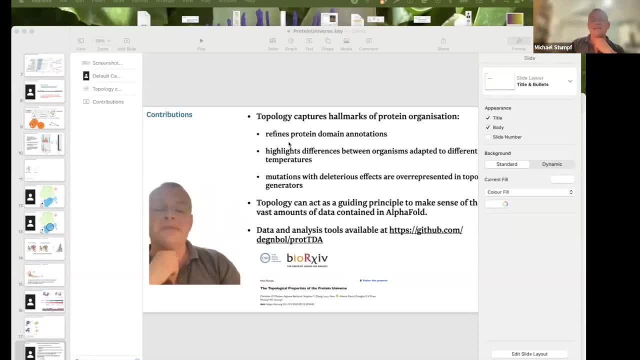 I hope that makes sense, And, Carol, so that seems to be the same question, So I hope that has now jointly answered this. Oh, so the point clouds what Nidhi asked. the point clouds are the 3D positions of the carbon alpha backbone atoms. 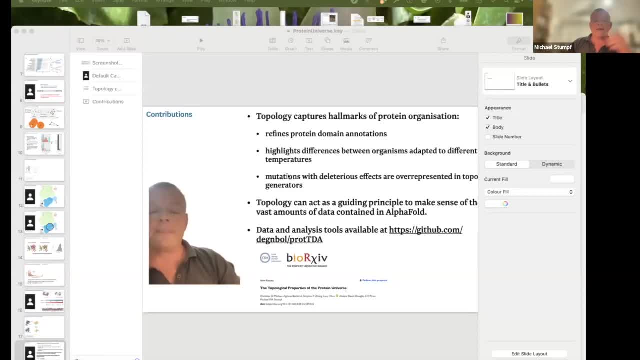 that we used to represent. We could have. we chose other things as well to compare, but that was our baseline to identify the mapping from the 3D structure into a point cloud. The next question is topological analysis applicable to analyzing protein structural ensembles. 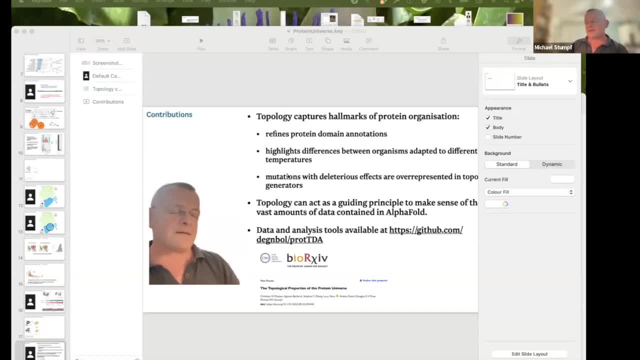 Yes, And you. there is work going on on making sure that we can identify this. We can define very nice distances between the topological structures, the features that we have or the hypergraphs that we use to represent them, And with that, you can, you can, you can do this analysis. 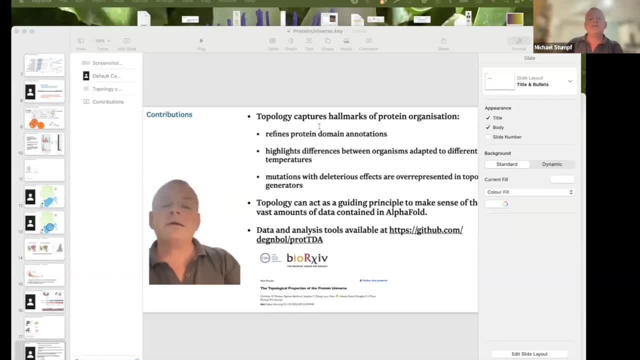 Are domains defined by topology? are not necessarily so. so space correct? Can you cluster domains at the scale of what Raymond Hackett asked? Are domains as defined by topology are not necessarily continuous in sequence, space correct? It's something which we worried about a lot More often than not when we looked at it. 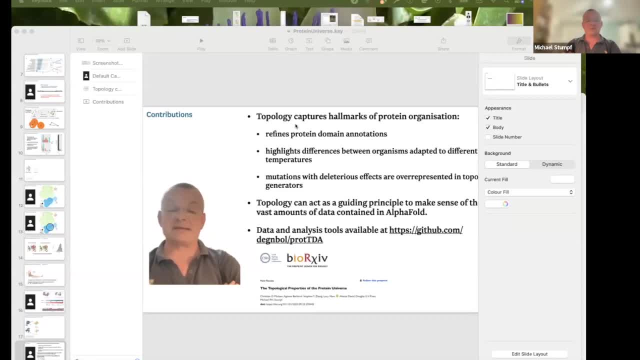 in sequence. there was still a distinction in sequence space as well. but they just they were inherited together, always in the cath database. but in our analysis we were able to identify different topological constituents. So you would never see them separate. but from a purely structured point of view it makes sense to say there is a difference. 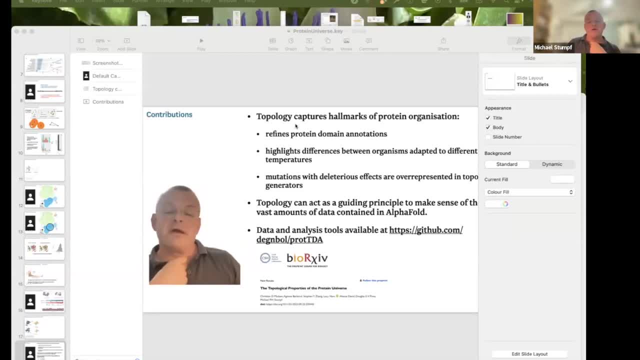 So I hope that goes somewhere to answering this. Mariana Watney says how sensitive are the topologies? Are topological features to a conformational state of the protein? Have you tried to write different conformations of the same protein? Yes, we have, and we used a very slow folding protein. 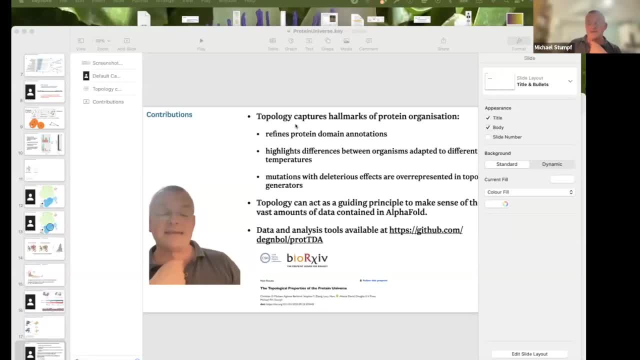 in the paper and tried to see if the topology generators correspond to those regions that are involved in the protein folding process. That's not quite the same as what you are after, I feel, but it's the closest that we we try to get to find some good data that allows us to test some changes in conformational state.